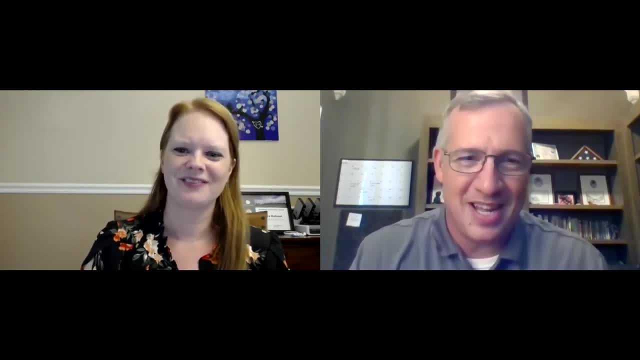 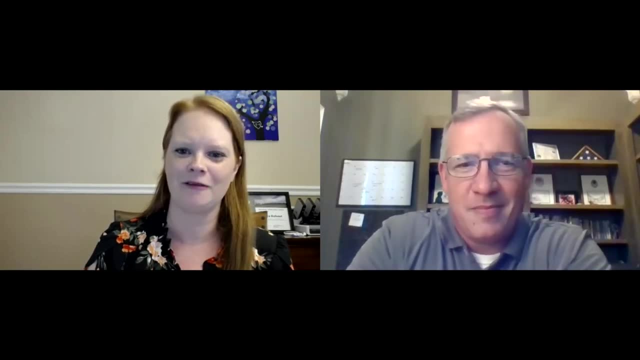 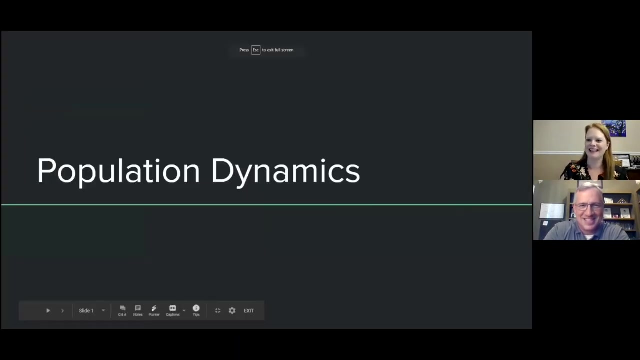 dynamics and how you're going to teach population dynamics to kids today. Sure, yes, population dynamics is a really cool biology concept, and why not learn about population dynamics by talking about zombies? So we're going to get into that a little bit like: how does that make sense? Well, 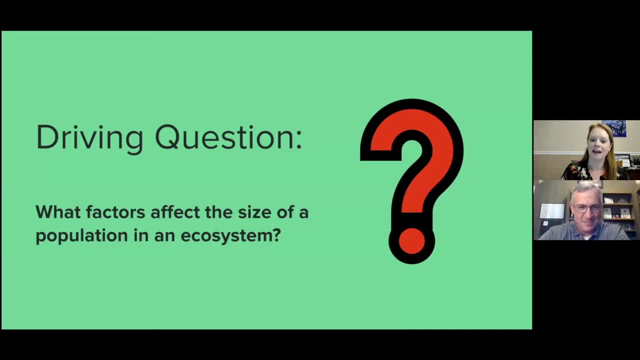 our driving question today are what factors affect the size of a population in an ecosystem. So if we think about zombies and the zombie apocalypse, we talk about how many zombies can a population hold, and so it's one of those things that might be really kind of fun and interesting and connect. 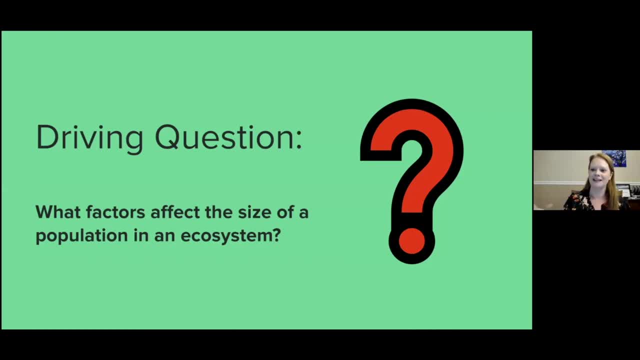 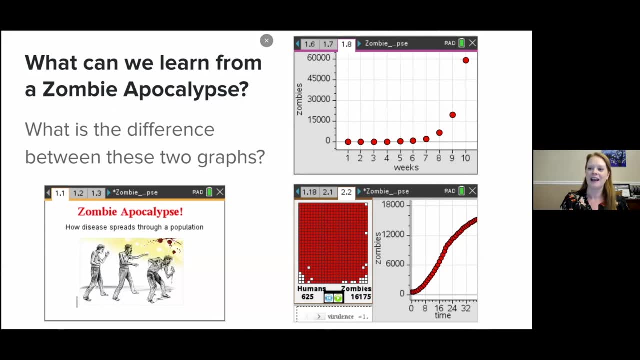 and then from there. maybe then students can apply it to situations in their own ecosystems, in their neighborhoods. But zombies are fun, and so here we have an example of the zombie apocalypse lesson from Stand Behind Hollywood, and I have two graphs: here and Eric, what is the difference between these two graphs? 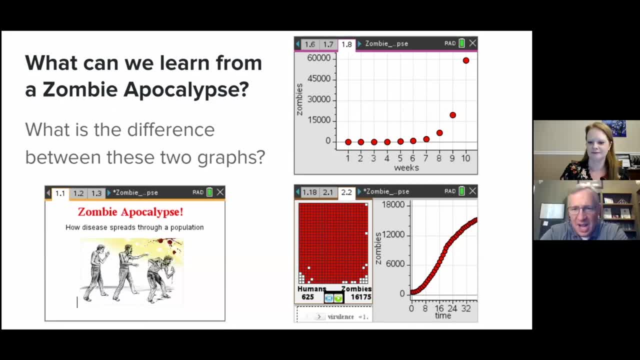 Well, let's see. so the top graph, the one that says zombies per weeks, it looks like the data is just sort of going up, like it looks like it just goes on forever. and then the graph below that, the data: it's zombies per time, whatever that unit of time is, and it looks like the data goes. 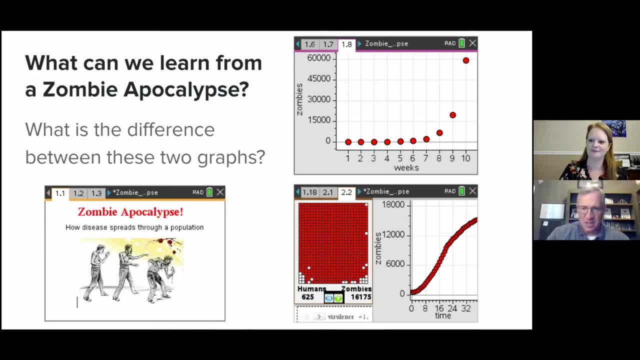 up, but then it starts to kind of flatten out a little bit. Is that the difference? Yeah, definitely, because it's a little bit more complex. The bottom graph, the two graphs at the top, it's just the population per week, So it's talking about a population per week, and then the Spanish. 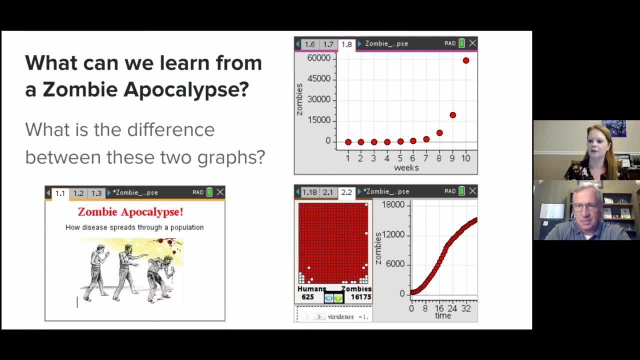 population per week and then the population per week. they're two different, so it's called the population per year for zombies. so it's all about population per year. So it's about how long a person is going to last, how long will they live, and then this graph is showing us how. 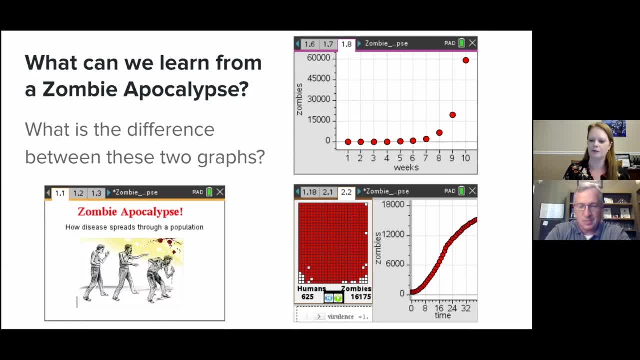 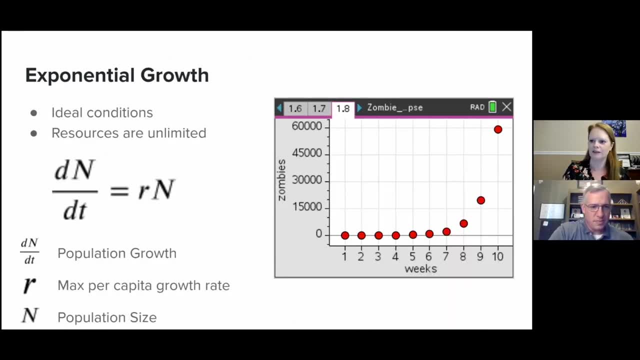 insane that population can be, how much human suffering it would cause. and again we can talk about that, the top of these specific types of graphs. so first let's talk about exponential growth, which is that first graph, and in this first graph, um, this is again in ideal conditions and unlimited resources. so 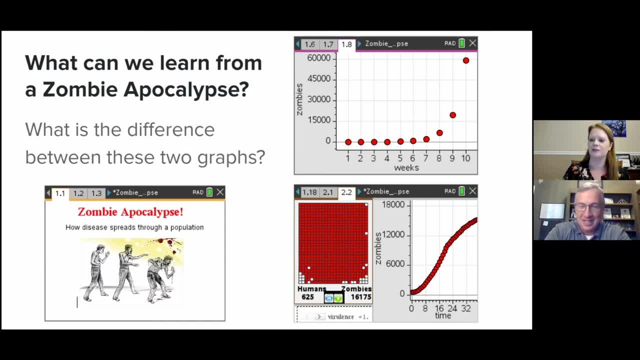 unlimited resources, their populations will continue to increase. and then the second graph at the bottom we have where zombies are. something about the population is causing the rate of increase to slow down, and we'll talk more about what's happening in each of these two graphs. 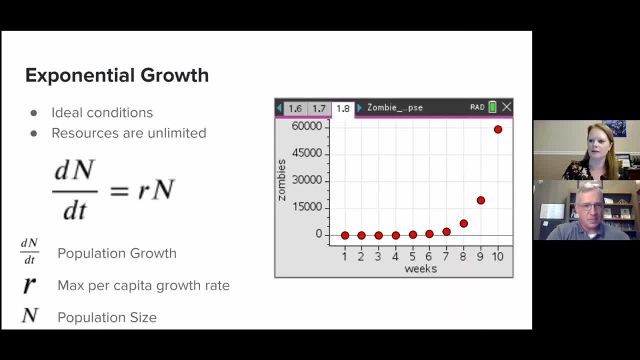 So first let's talk about exponential growth, which is that first graph. and in this first graph this is again in ideal conditions and unlimited resources. So if we're talking about zombies, what are the things that zombies need? When you say resources, do you mean humans? that? 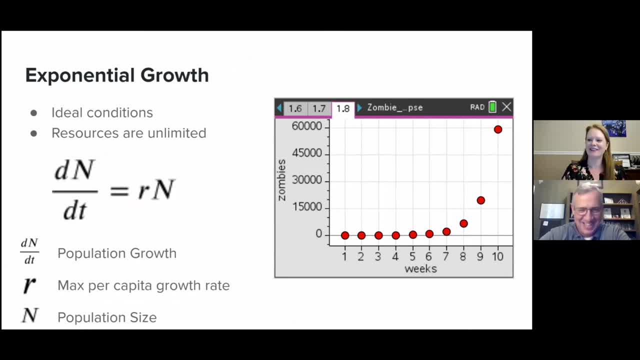 they eat. Yes, they need food. So food is a resource, and so if zombies' populations are increasing, they're eating food. So if zombies' populations are increasing, they're eating food. They have unlimited resources and plenty of humans to munch on, and so, in this case, we have a time. 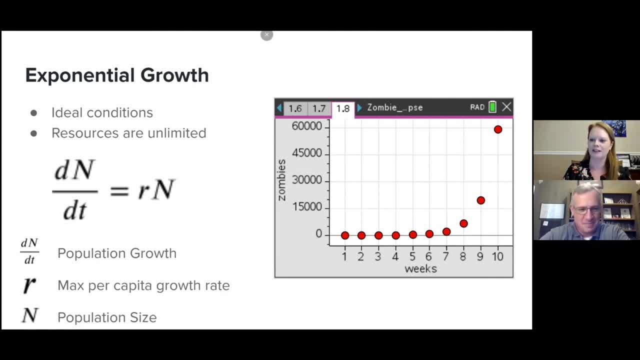 range of about 10 weeks, and our zombie population is increasing, and right now it's, you know, getting close to about 60,000 in 10 weeks, and so we're going to apply an equation of the change in the population over. the change in time is going to equal the max per capita growth rate times the. 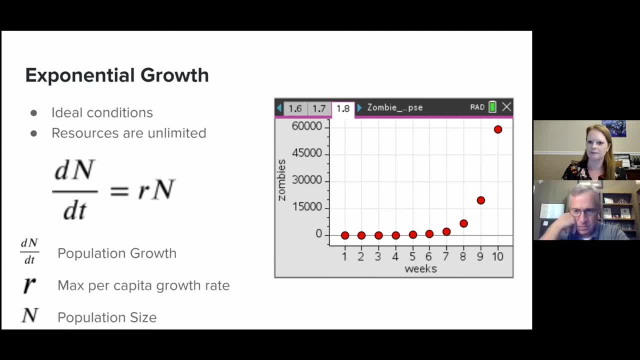 population size. So we're going to apply an equation of the change in the population over. the change in time is going to equal the max per capita growth rate times the population size. So we're going to be playing with this equation a little bit later on. but I wanted to highlight this equation because 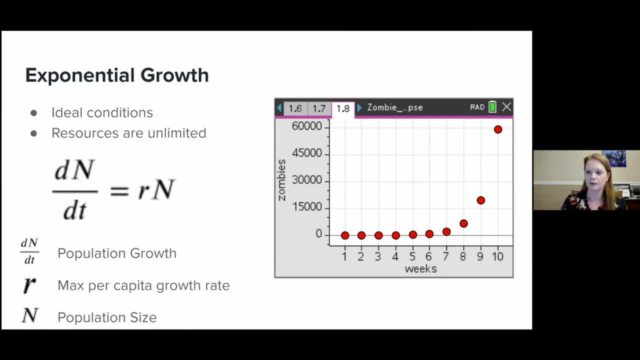 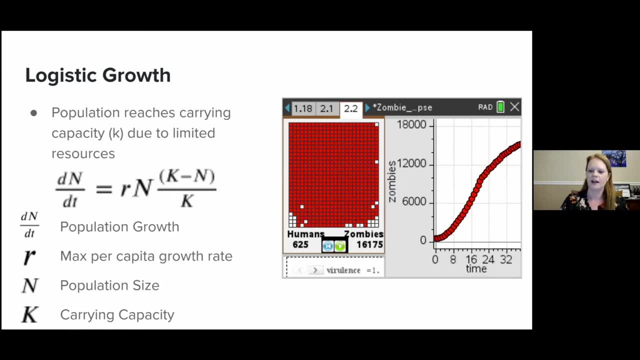 that's going to help us understand how the population grows, and we're going to be applying it to zombies in this case. So the other type of growth is logistic growth, and so that's where we saw that initial increase and then that rate levels off, and so this is where our population 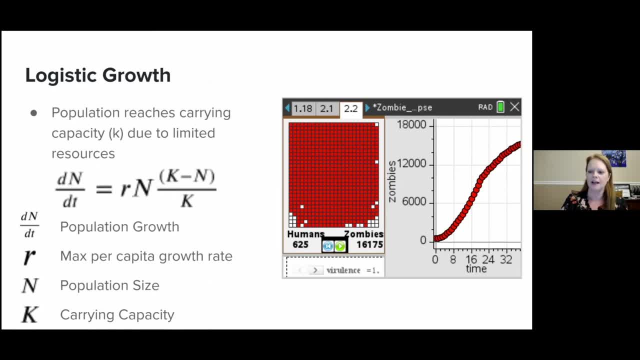 reaches what is called a carrying capacity, and so carrying capacity is that limit in which the population reach reaches. where it can't be successful. past that number, It's that those birth rates start to decrease and the death rate starts to increase, and so you're running out. 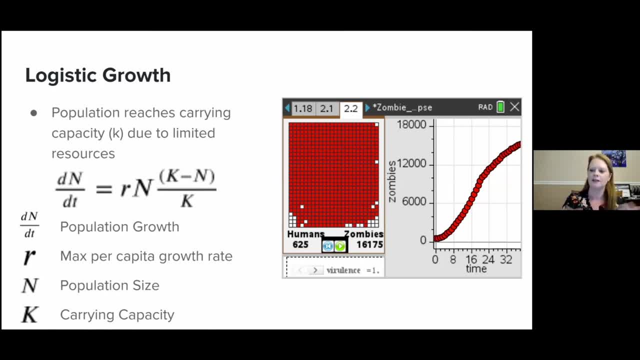 of those resources. That's the cap of those resources. So what are the zombies running out of? Well, I don't know if this is a good or bad thing, but they're running out of healthy people to eat. Yeah, they're running out of that food resource. So you see that. 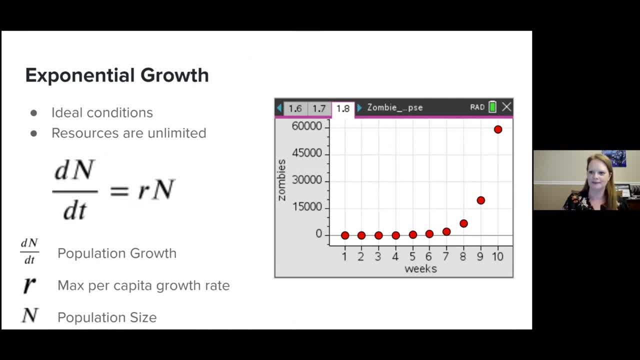 if we're talking about zombies. what are the things that zombies need? when you say resources, do you mean humans that they eat? yes, they need food, so food is a resource, and so if zombies populations are increasing, they're eating their food. they have unlimited resources and plenty of humans. 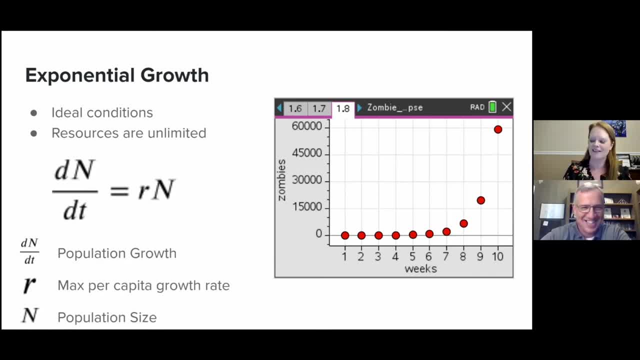 to munch on. and so in this case, we have a time range about 10 weeks and our zombie population is increasing, and right now it's, you know, close, getting close to about 60 000 in 10 weeks. and so we're going to apply an equation of the change in the population over the change in time. 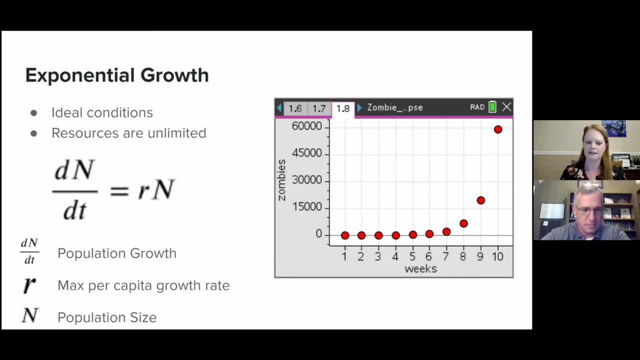 is going to equal the max per capita growth rate times the population size. so we're going to be playing with this equation a little bit later on, but i wanted to highlight this equation because that's going to help us understand how the population grows, and we're going to be applying it to zombies in this case. so the other type of 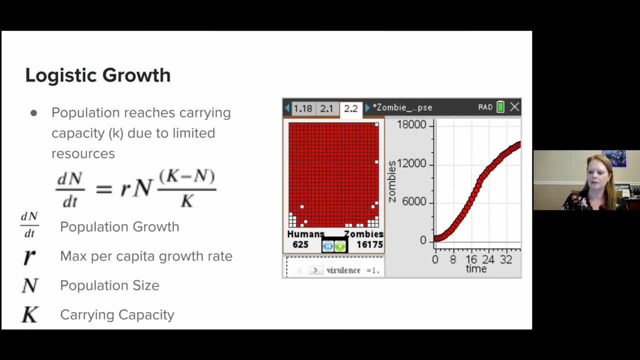 growth is logistic growth, and so that's where we saw that initial increase and then that rate levels off, and so this is where our population reaches what is called a carrying capacity, and so carrying capacity is that limit in which the population reach, reaches where it can't be. 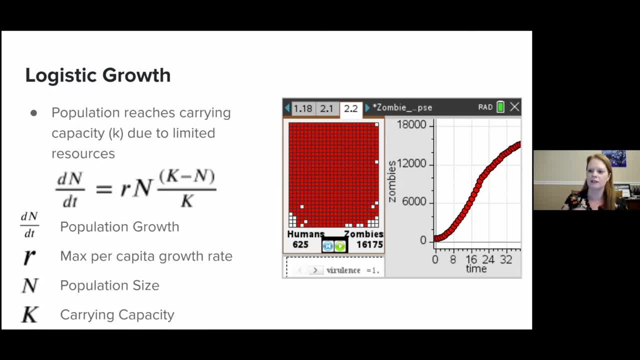 successful past that number. it's that those birth rates start to decrease, um and the death rate starts to increase. so you're running out of those resources. that's the cap of those resources. so what are the zombies running out of? well, i i don't know if this is a good or bad thing. 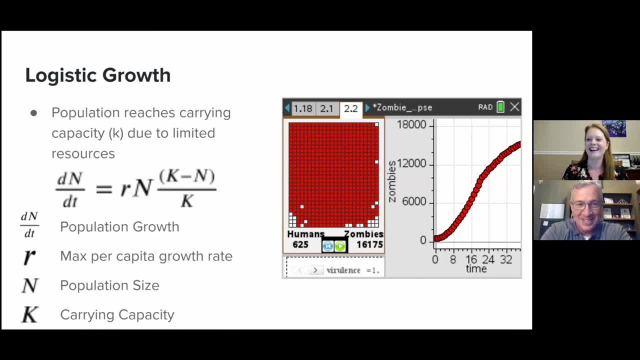 but they're running out of healthy people to eat. yeah, they're running out of that food resource for. so you see that they're reaching that carrying capacity based off of the amount of food that's available and that's represented as k, and so we take that um, that max per capita growth rate, and 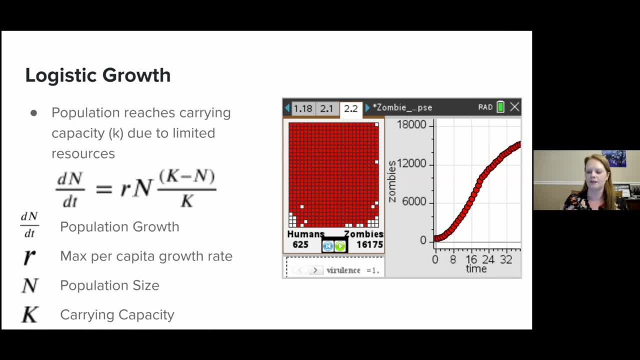 that population size and we multiply it by this proportion of carrying capacity, of carrying capacity minus the population over carrying capacity. and so if we think about those values, if our population or n is very small and our carrying capacity is very high, then our rate is going to be closer to one and we're going to be 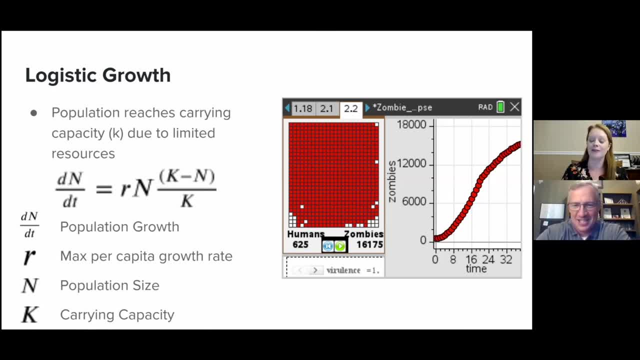 they're reaching that carrying capacity based off of the amount of food that's available and that's represented as K. and so we take that max per capita growth rate and that population size and we multiply it by this proportion of carrying capacity minus the population over. 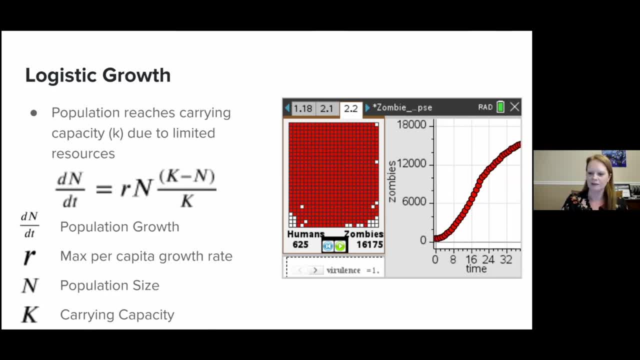 carrying capacity. and so, if we think about those values, if our population or N is very small and our carrying capacity is very small, then we're going to have a population that's very small, and if our population or K is very high, then our rate is going to be closer to one and we're going 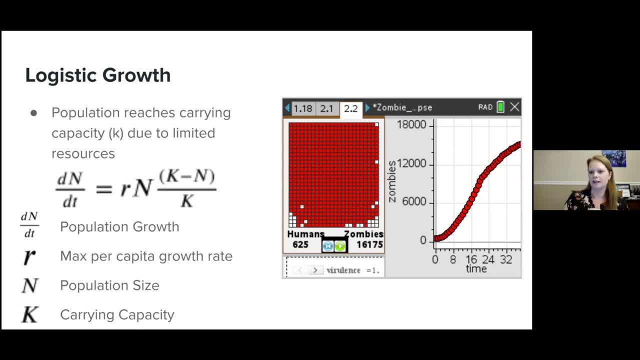 to be increasing very quickly. but as that number, as that population number, N, gets higher and our carrying capacity, carrying capacity or K- gets closer, or that N gets closer to that K, it's going to be closer to zero. and oops, and that's where you're going to be leveling out in this top. 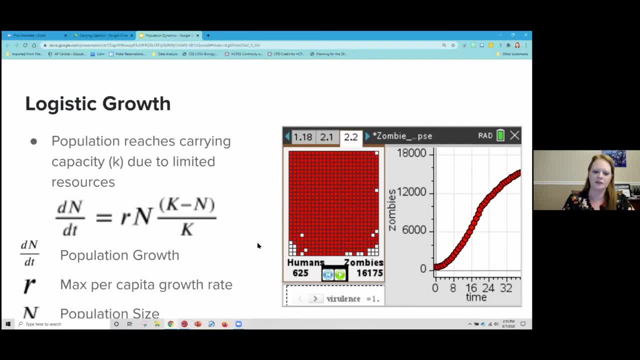 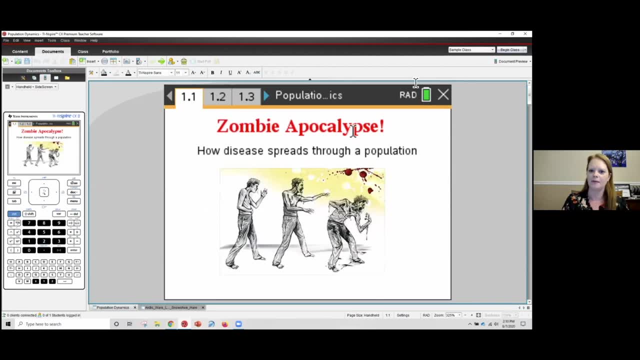 bar here, and so we're going to play around with some of these graphs so that we can hopefully make sense of it, And so I pulled some of these graphs from the zombie apocalypse activity on STEM Behind Hollywood and just for my personal use in terms of this video, to show you some of those really. 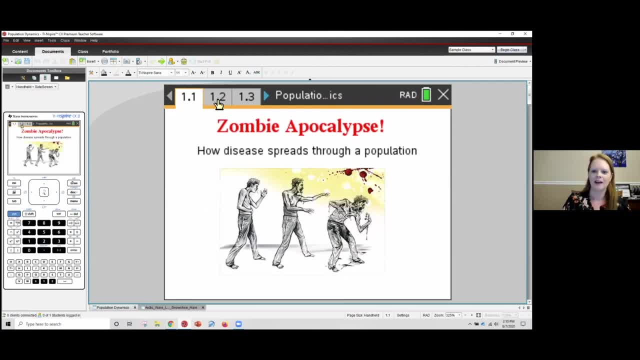 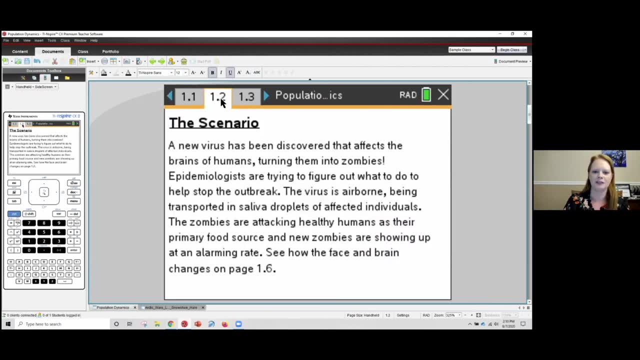 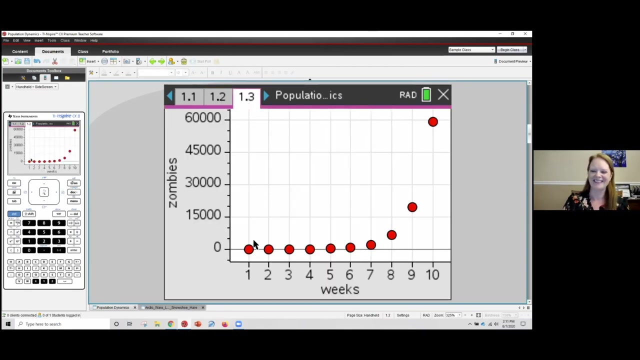 cool graphs in terms of exponential and logistic growth, and so you can kind of see the stages of the zombie as it goes and becomes our full zombie population. and in this activity, this, zombies are formed. They're formed by a virus that's transmitted through air droplets, so it's a little close to home right now. 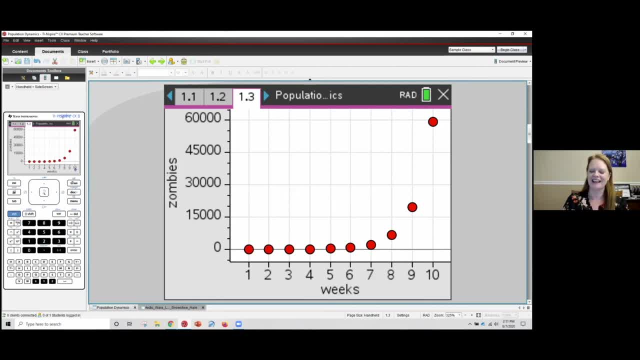 And so what we see in this graph is that same one from before. so over 10 weeks we see this increase of our zombie population, and then in the next graph here I'm going to show you, it's just going to be a. 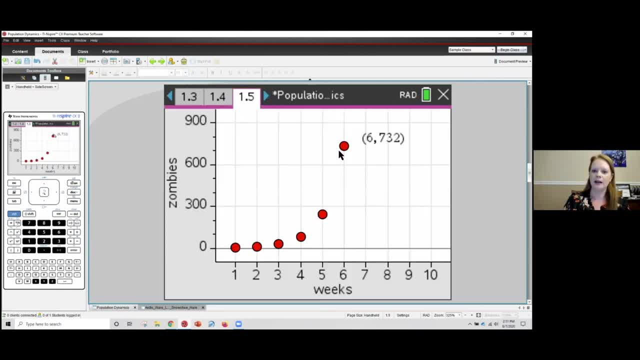 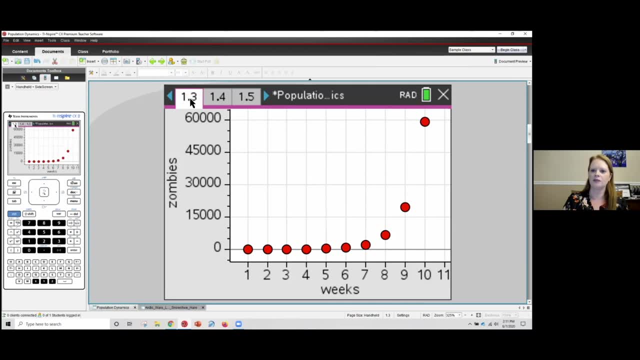 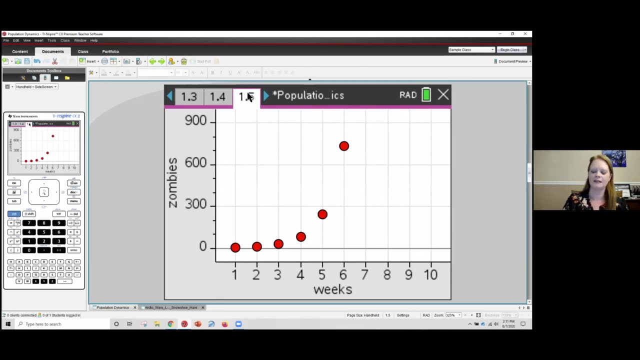 different scale. So it's still 10 weeks, but we're not done yet. We're not done yet. So it's still 10 weeks, but now we're only looking at around 700 in terms of our population. So if we compare to our 60,000 zombies versus our 9 or less than 900 zombies, we see this big change in scale. 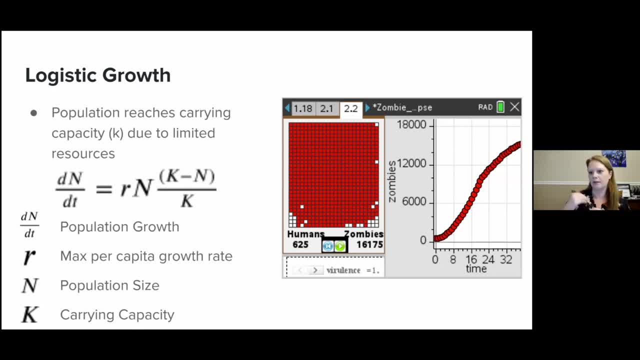 increasing very quickly. but as that number, as that population number n, gets higher and our carrying capacity, carrying capacity or k gets closer, or that n gets closer to that k, it's going to be closer to zero. and oops, and that's where you're going to be leveling out in this top bar. 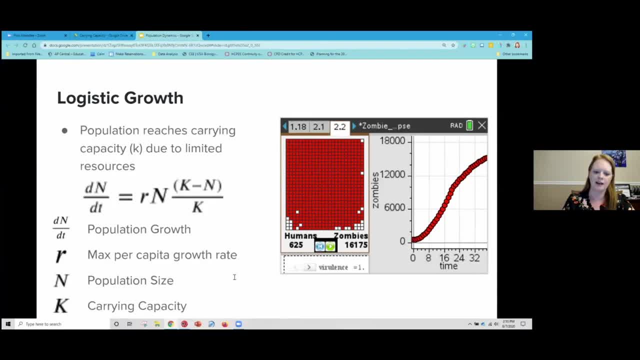 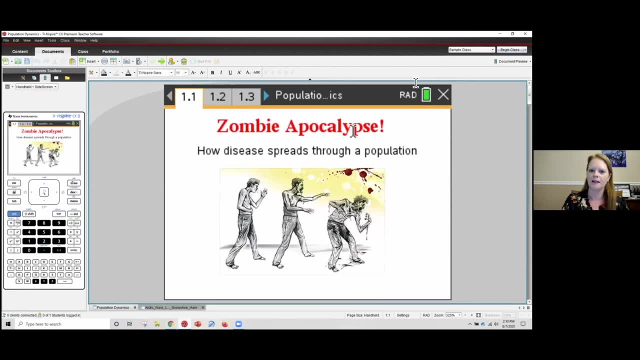 here, and so we're going to play around with some of these graphs so that we can- hopefully I'll show you one of my videos where i talk about this with you in further introduction, so you can see all these datas and how I use them to help you make sense of it. 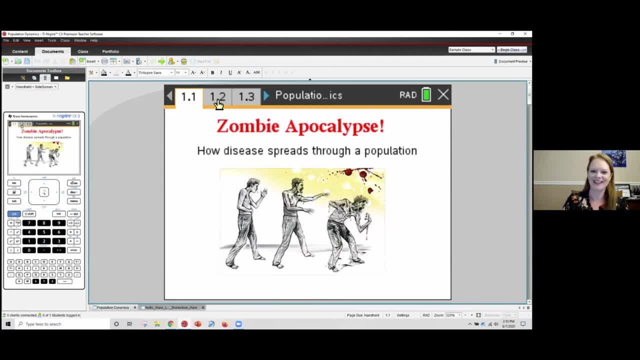 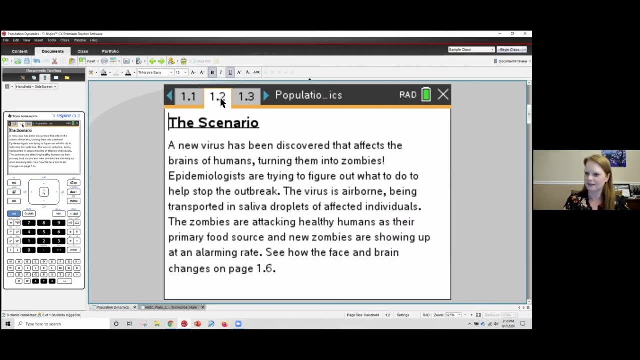 and so I've pulled some of these graphs from the zombie apocalypse activity on stem behind Hollywood and just for my personal use in terms of this, this video, to show you some of those really cool graphs in terms of exponential and logistic growth, and so you can kind of see the 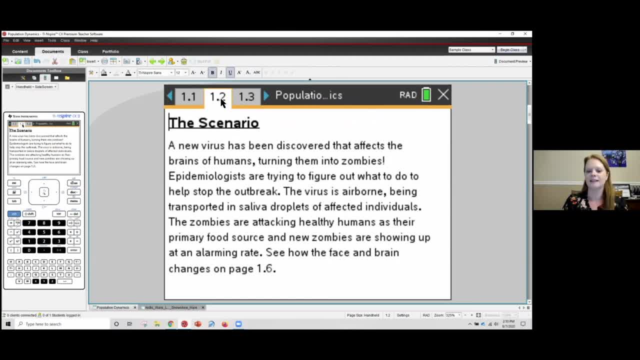 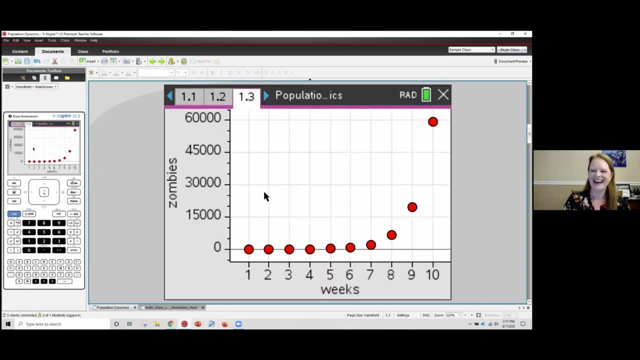 Zombies are formed by a virus that's transmitted through air droplets. So it's a little close to home right now, And so what we see in this graph is that same one from before. So over 10 weeks we see this increase of our zombie population. 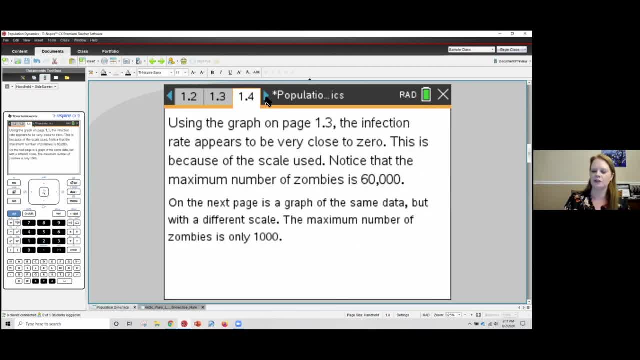 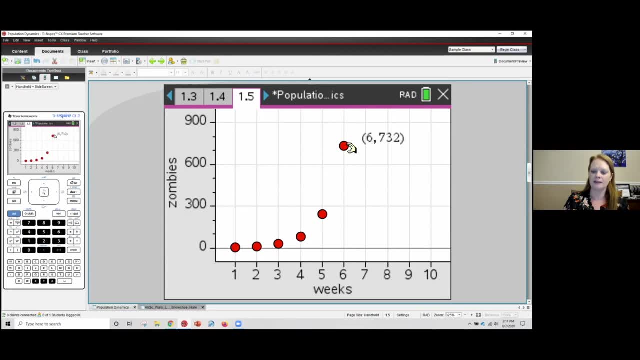 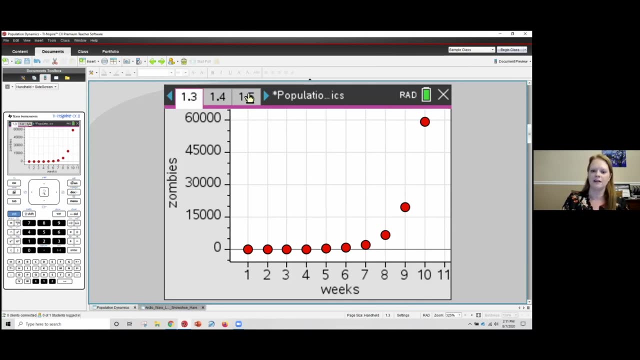 And then in the next graph here I'm gonna show you. it's just gonna be a different scale. So it's still 10 weeks, but now we're only looking at around 700 in terms of our population, If we compare to our 60,000 zombies. 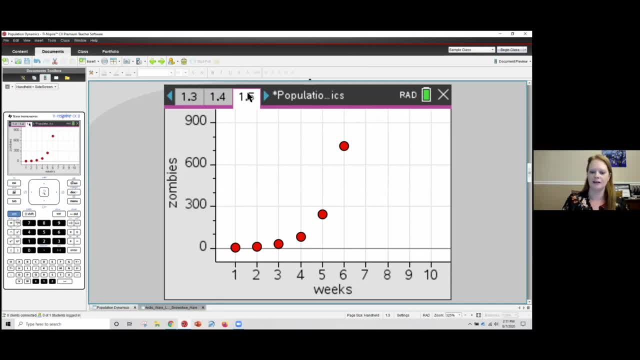 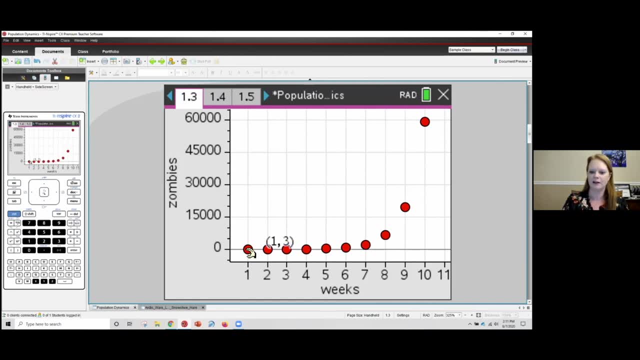 versus our nine or less than 900 zombies. we see this big change in scale, And so here in this first few weeks, week one through six- it doesn't seem like it's growing too much, But when you're really looking at it, 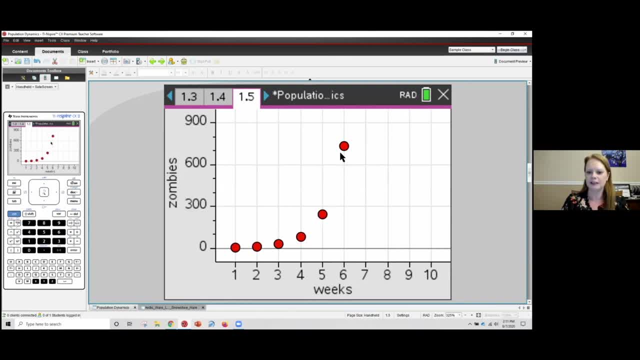 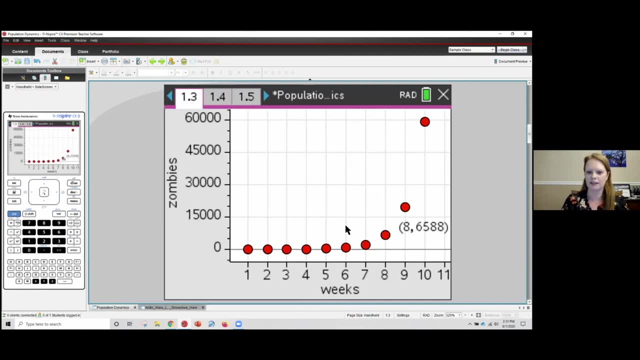 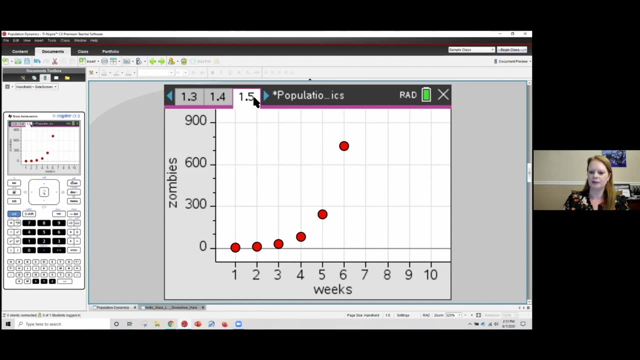 a little bit more closely. that rate is really increasing at a much well, it's the same rate as here, but it just appears visually to be faster, And so getting approaching the data at a different scale is really important for students to visualize how these values change. 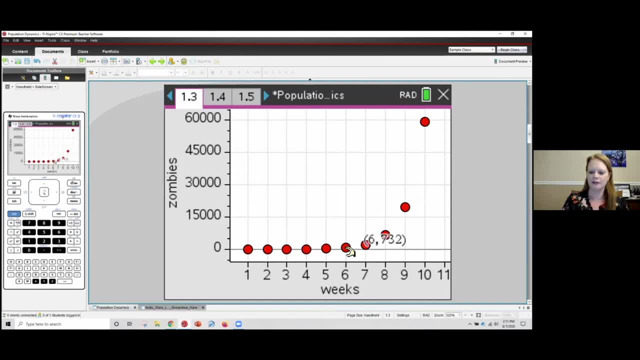 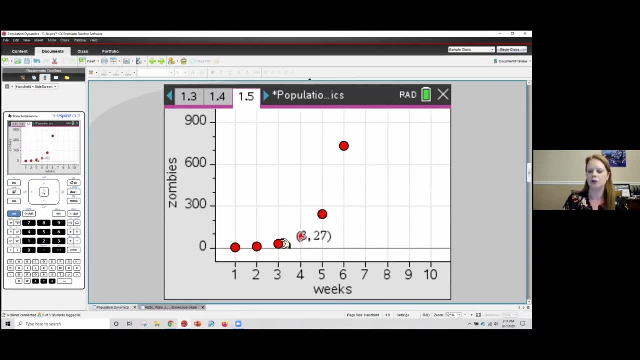 And so here in this first few weeks- week one through six- it doesn't seem like it's growing too much. but when you're really looking at it a little bit more closely, that rate of growth is going to be a little bit higher. 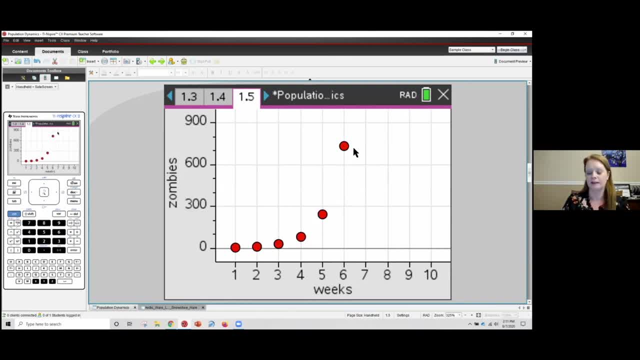 That rate is really increasing at a much. well, it's the same rate as here, but it just appears visually to be faster, And so getting approaching the data at a different scale is really important for students to visualize how these values change. 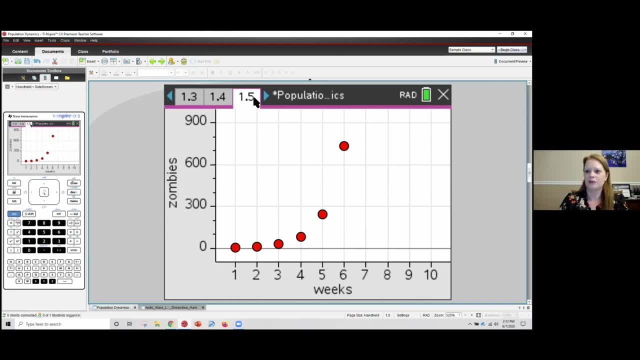 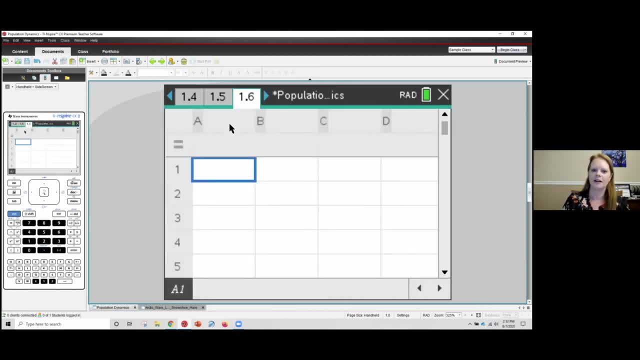 And so what I like to do also is to put this information in a spreadsheet so they can play with it, And so I put in a spreadsheet here where I'm going to show you the data, I'm going to show you the data, I'm going to show you the data. 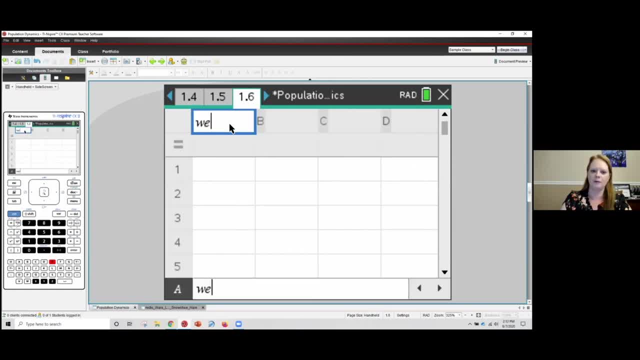 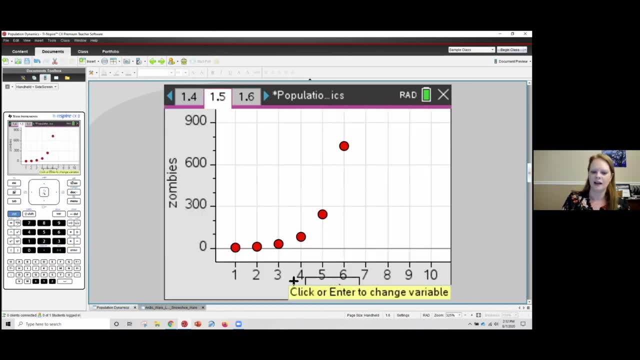 So I'm going to be looking at our week And that's going to populate because that was in the previous chart here. And then our first week we had three zombies. We look at that ordered pair, It's one, three. So at week one we have three zombies. 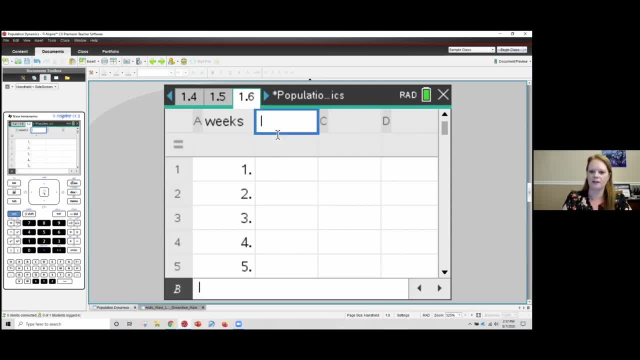 So I'm just going to put that from that equation: r times n, And I'm going to get rid of this right now, And so that's our first one in three. But I want to populate the rest of my chart by adding in an equation: 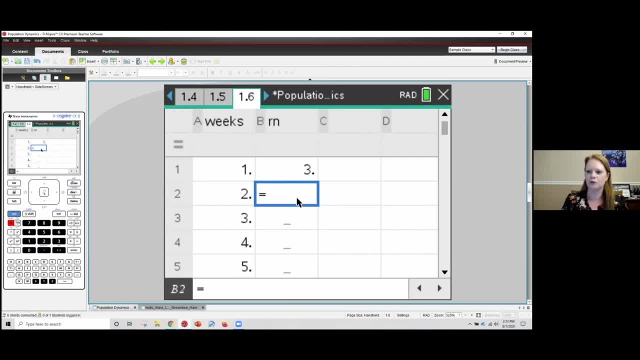 And so using spreadsheets is this great computational tool that students should have experience with, And so I like to show students how to add equations to a spreadsheet in order to help them understand the data that they're collecting. And so what I'm doing here is I'm going to take this value so that first week, and then I'm going to multiply it. 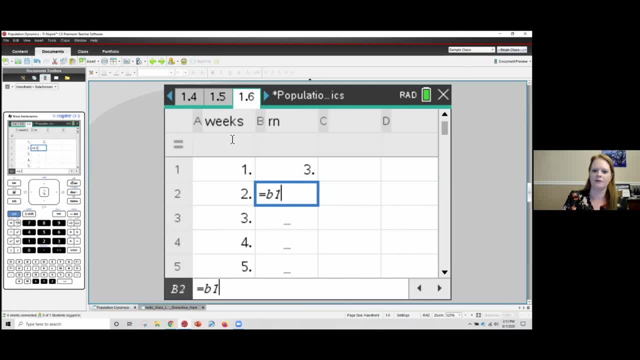 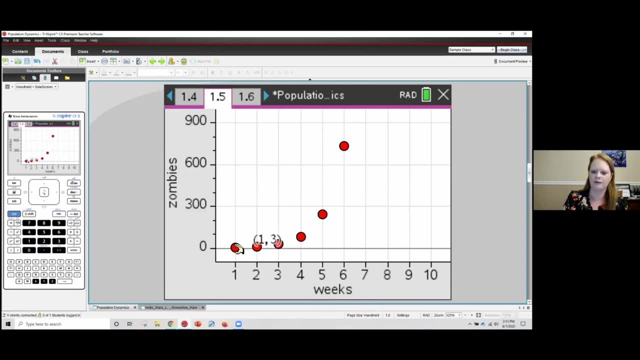 So this is our n right now, And I'm going to multiply it by the rate, And so we can find the rate by looking at these values. So we have got one. At week one we've got three zombies, And at week two we have nine zombies. 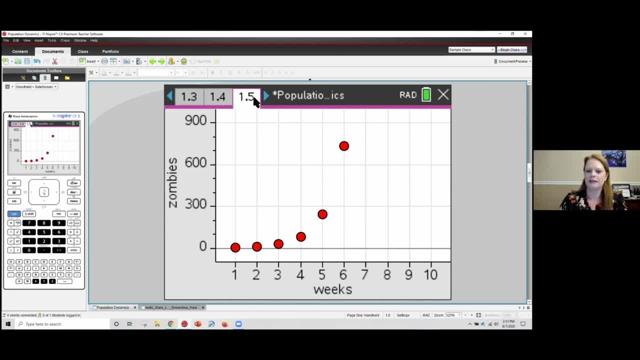 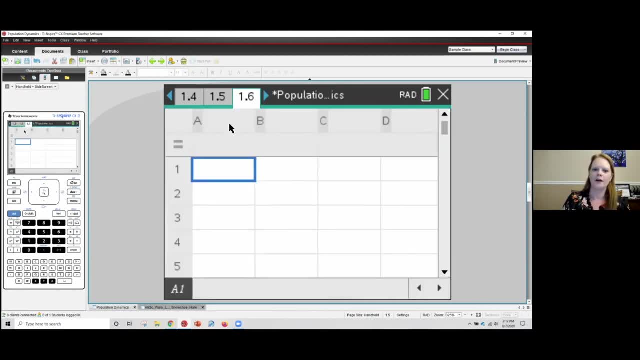 And so what I like to do also is to put this information in a spreadsheet so they can play with it, And so I put in a spreadsheet here where I'm going to be looking at our week, And that's gonna populate, because that was in the previous chart here. 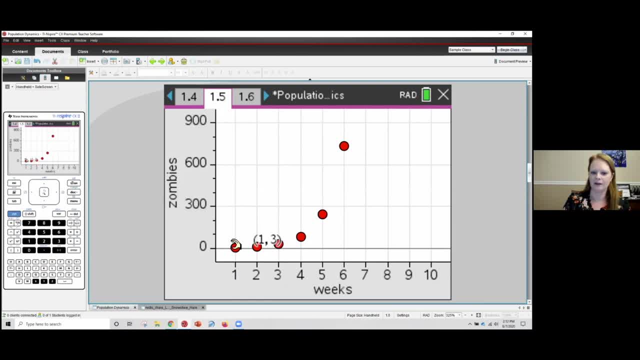 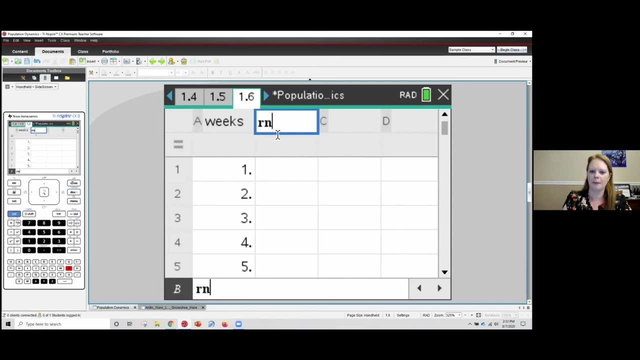 And then our first week we had three zombies. We look at that ordered pair, it's one, three. So at week one we have three zombies. So I'm just gonna put from that equation R times N, And I'm going to get rid of this right now. 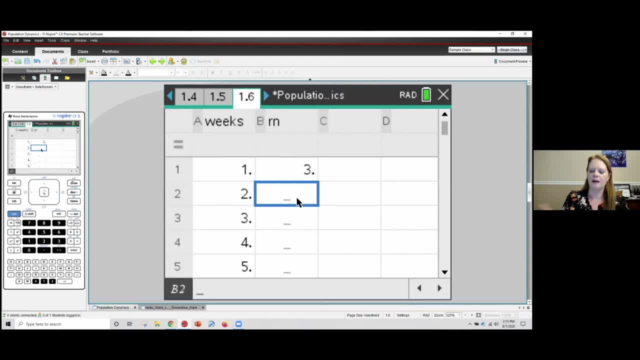 And so that's our first one and three, But I wanna populate the rest of my chart by adding in an equation, And so, using spreadsheets, is this great computational tool that students should have experience with, And so I like to show students how to add equations. 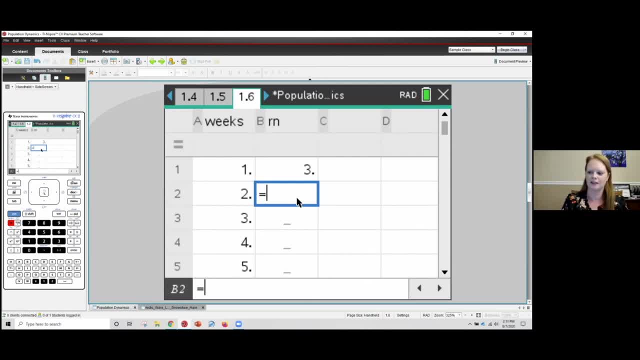 to a spreadsheet in order to help them understand the data that they're collecting. And so what I'm doing here is I'm gonna take this value so that first week, and then I'm gonna multiply it. So this is our N right now. 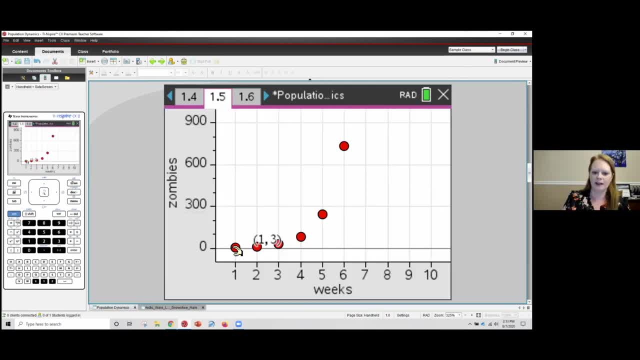 and I'm gonna multiply it by the rate, And so we can find the rate by looking at these values. So we have got one. at week one we've got three zombies, and at week two we have nine zombies. So what is our change in zombies? 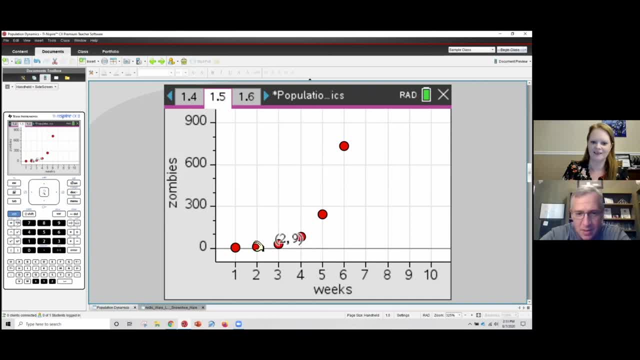 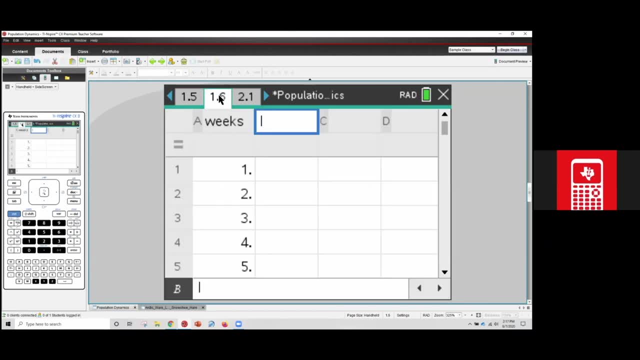 So the increase in what we're talking about is obviously the increase in the rate of sex activity. And so in week one, 100 times over, we are collecting organ count numbers. So this is what we're had in week one, And then we're adding the rate to. we have major students. 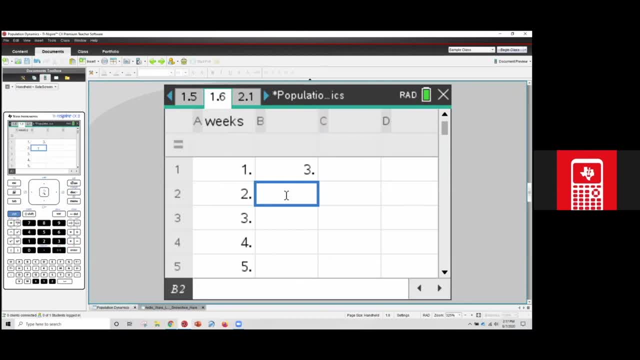 in week two, three, And we have a reason for sure, because last week we looked back on theש, where six zombies were added in one week. Right, and so six zombies were added in one week. But we can take this and put it in a spreadsheet, So we have the week. We can then look at the ratesに. 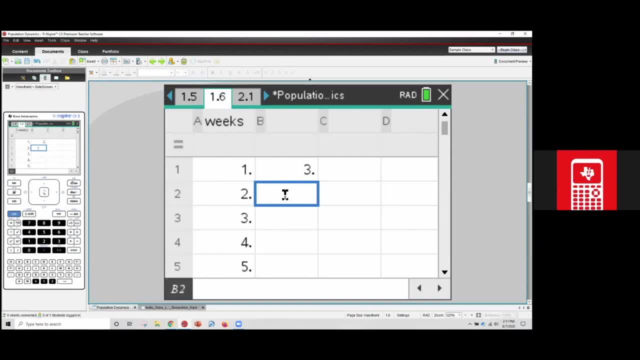 So if we're starting out with three zombies, then we can then add in an equation And to give students an opportunity to play with spreadsheets, manipulate spreadsheets and understand what's going on, but to by playing with some of these numbers and using equations to represent what's. 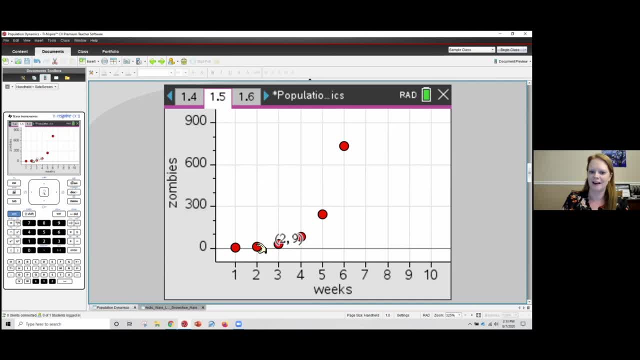 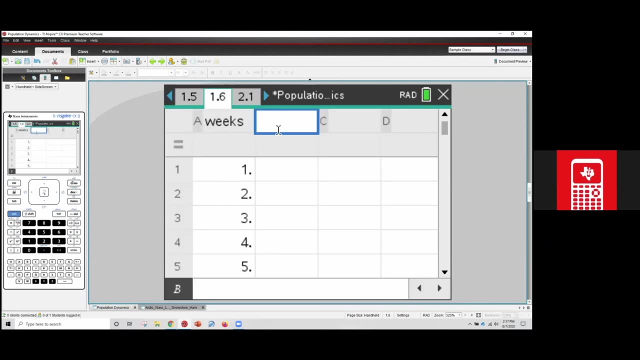 So what is our change in zombies? Six zombies were added in one week, Right, And so six zombies were added in one week. So we can take this and put it in a spreadsheet. So we have the week. We can then look at the rate. 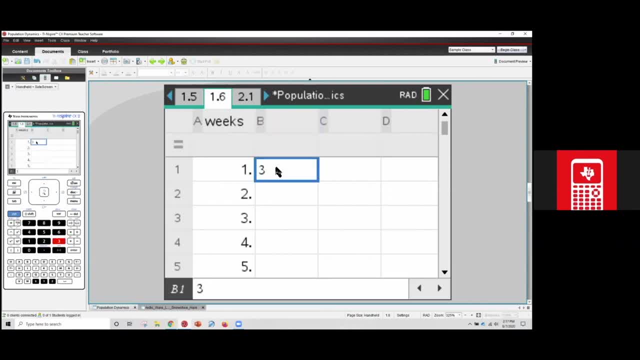 So if we're starting out with three zombies, we can then add in an equation, And I feel it's really important to give students an opportunity to play with spreadsheets, manipulate spreadsheets And understand what's going on by playing with some of these numbers and using equations to represent what's happening. 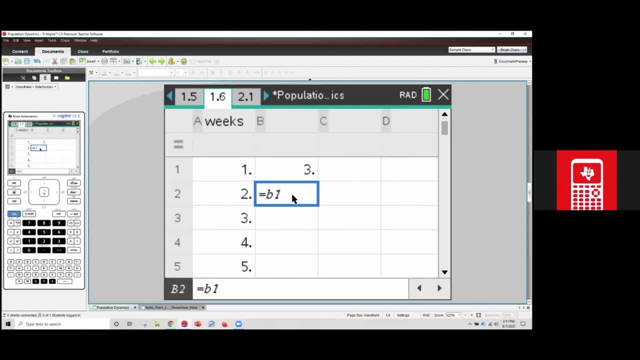 And so if three is our first zombie, we're going to take that first zombie. So I'm going to click on B1 to represent our first week of zombies. We had three, And then we're going to multiply that by the rate. 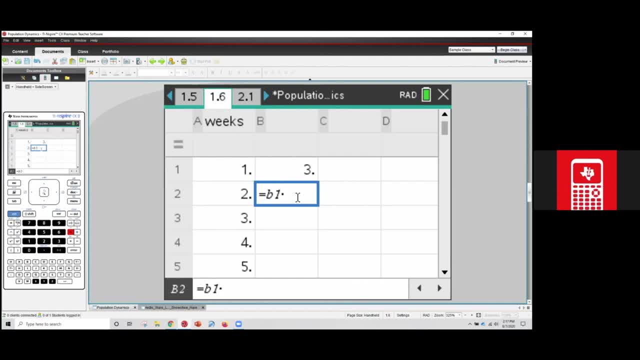 So it's r times n, And so this is our n, So our r. Let's start with three, And that would give us nine, And so we can then drag this then down to see how that would affect how many zombies we would create in a given period of time. 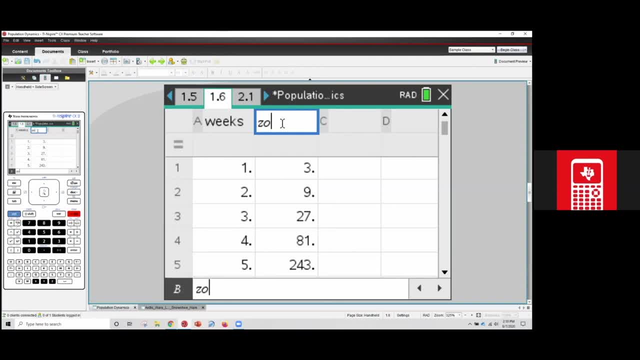 Or I should say zombie n. We'll name it that, And so if I move down a little bit further, I'm going to drag this all the way down to. we have now nine, I think it was 10. And then we can use this spreadsheet to make another graph. 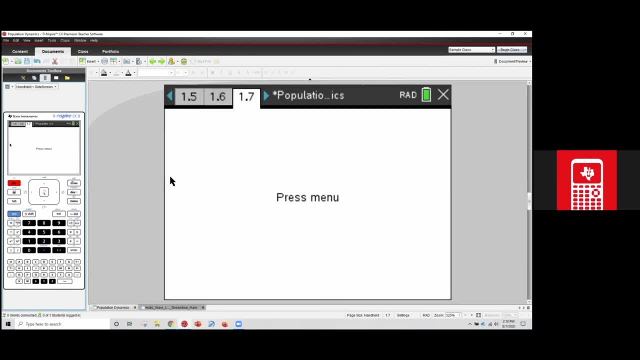 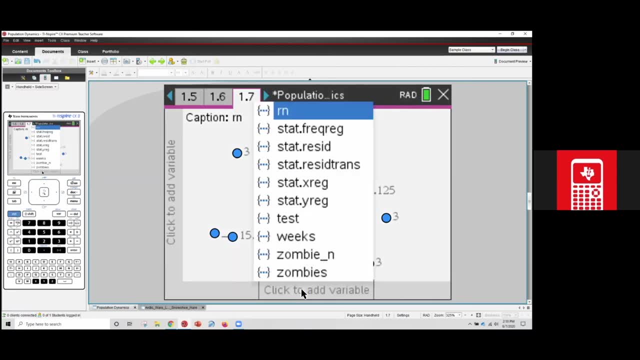 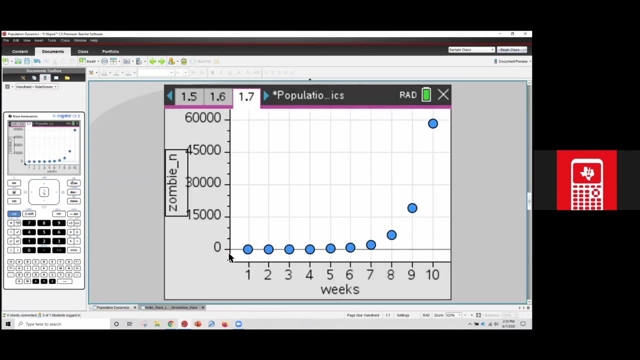 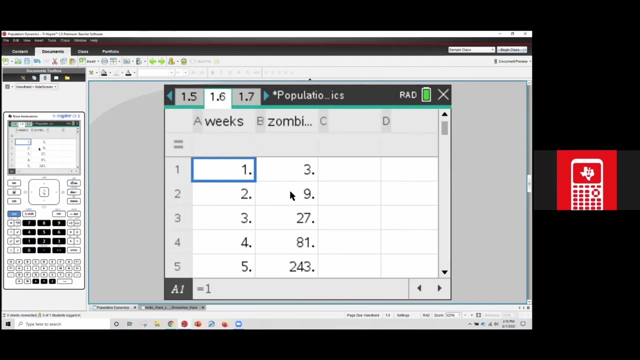 So I'm going to hit control and doc, There it was. And then I'm going to add a data and statistics page And I'm going to graph our weeks Versus our zombies n to see how our exponential growth works. I can also then go and change what happens here. 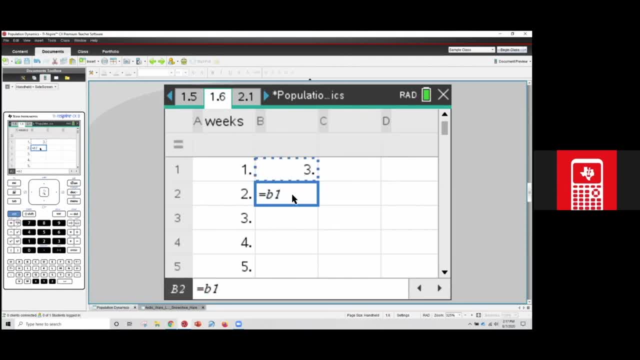 happening, And so if three is our first zombie, we're going to take that first zombie. so I'm going to click on B1 to represent our first weeks of zombies. we had three, and then we're going to multiply that by the rate, so it's R. 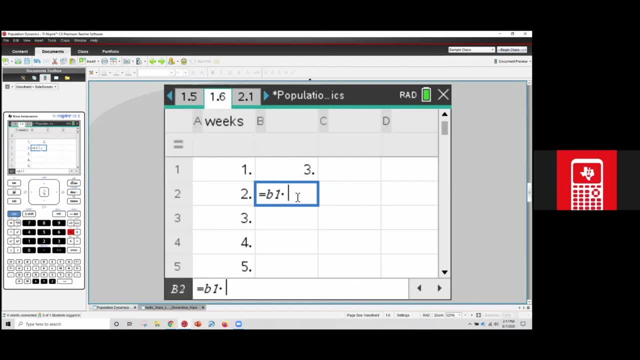 times N, And so our. this is our N, so our R. let's start with three, and that would give us nine, And so we can then drag this then down to see how that would affect how many zombies we would create in a given period of time, Or I should. 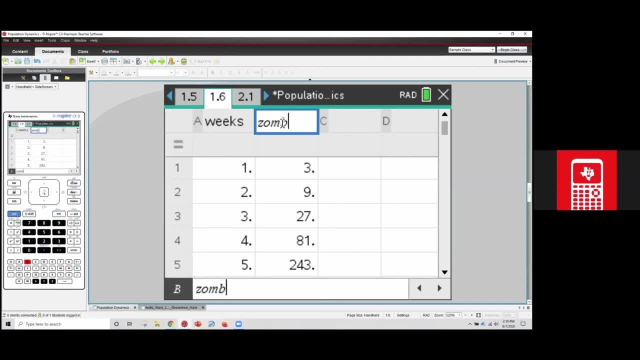 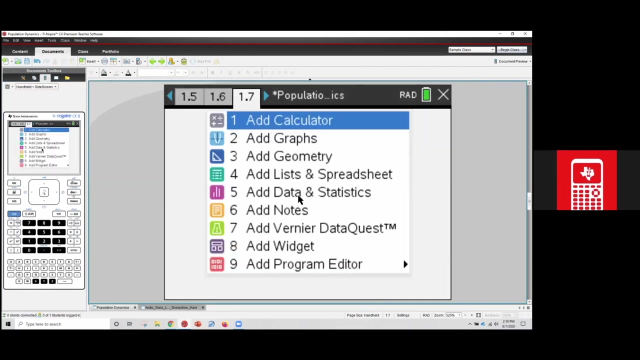 say zombie, I'll do N. We'll name it that, And so if I move down a little bit further, I'm gonna drag this all the way down to we have now, and then we can use this spreadsheet to make another graph. so I'm going to hit ctrl and dock- there I was, and then I'm going to add a. 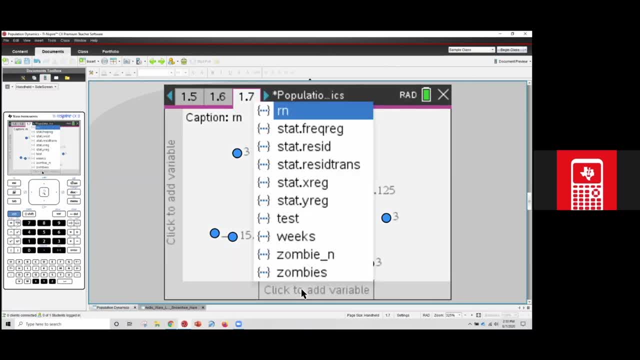 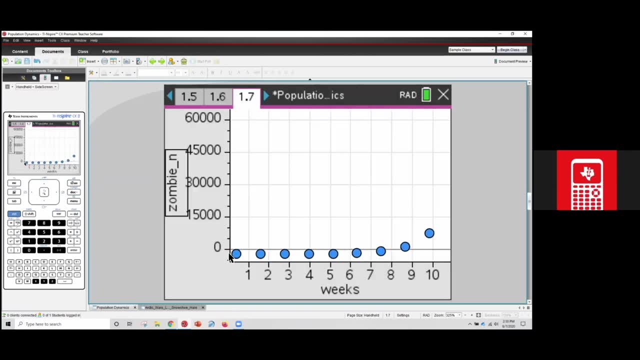 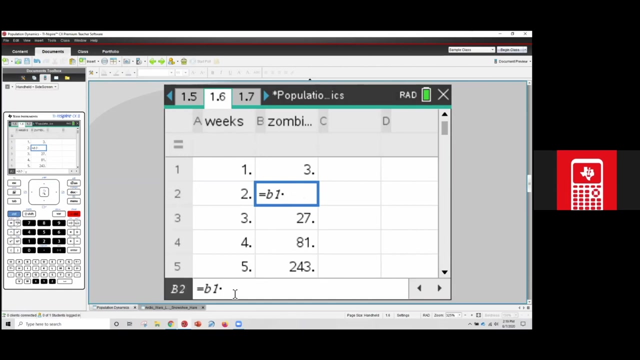 data and statistics page And I'm going to graph our weeks versus our zombies end to see how our exponential growth works. I can also then go and change what happens here. So let's say, our zombie are increasing at a much higher rate. So 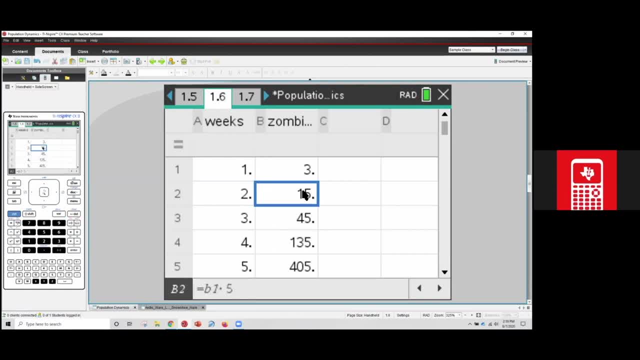 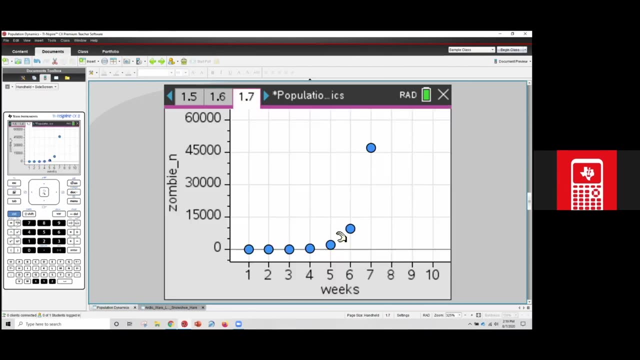 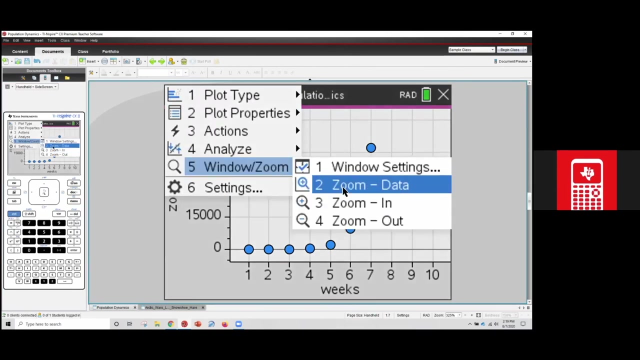 let's say, at five, And so we can take this and drag this down, That last one, And it increased significantly And we can see that in our graph here as well. So actually I need to zoom on our data. We're not even seeing all of it right now. So if I zoom in our data, our zombie numbers have. 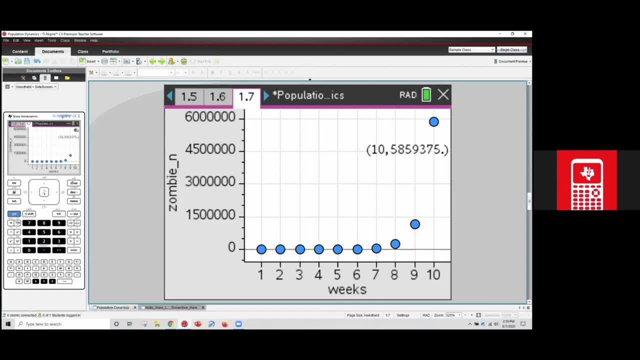 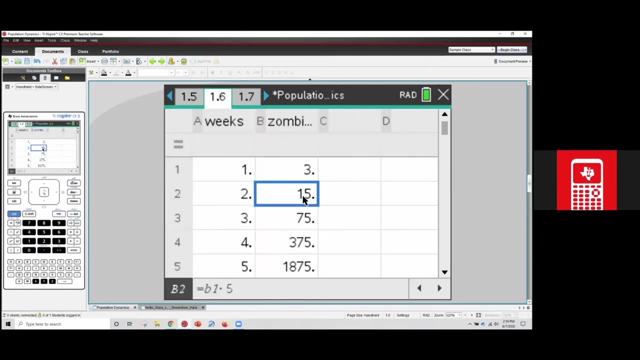 increased quite a bit. So we went up. I think our max was around 60,000.. And now we're pushing up to 6 million. So by changing the rate and looking at what's happening here, we're seeing a much bigger number based on. 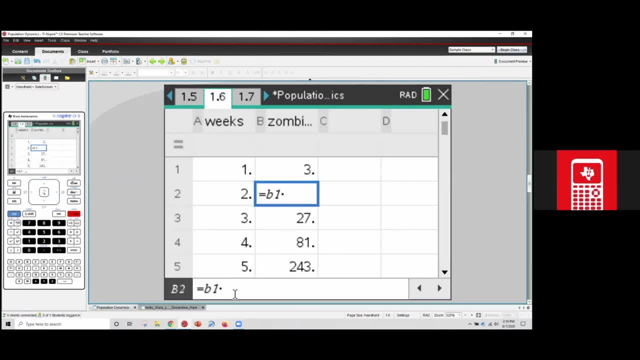 So let's say, our zombies are increasing at a much higher rate, So let's say at five, And so we can take this and drag this down Too far, And we can see that our zombie numbers have increased significantly, And we can see that in our graph here as well. 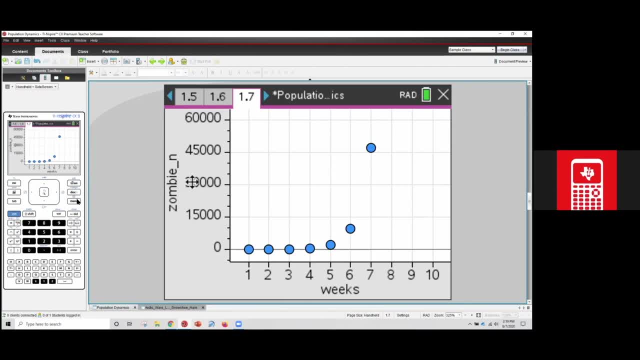 So actually I need to zoom on our data. We're not even seeing all of it right now. So if I zoom in our data, our zombie numbers have increased quite a bit. So we went up. I think our max was around 60,000.. 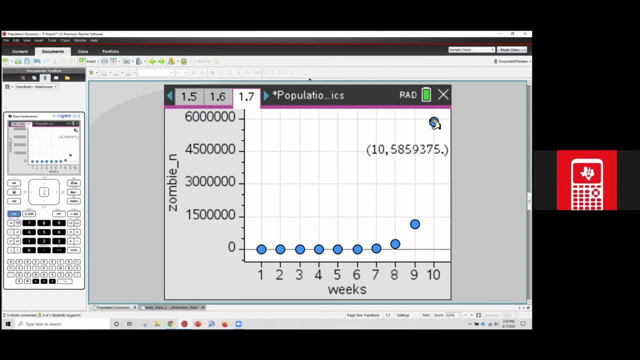 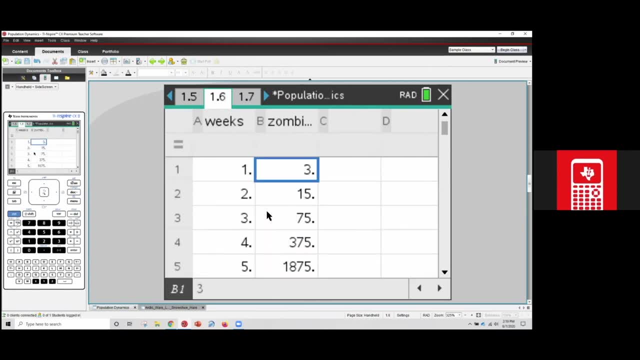 And now we're pushing up to 6 million. So by changing the rate and the number of zombies And by changing the rate and looking at what's happening here, We're seeing a much Bigger number based on how the rate changes. 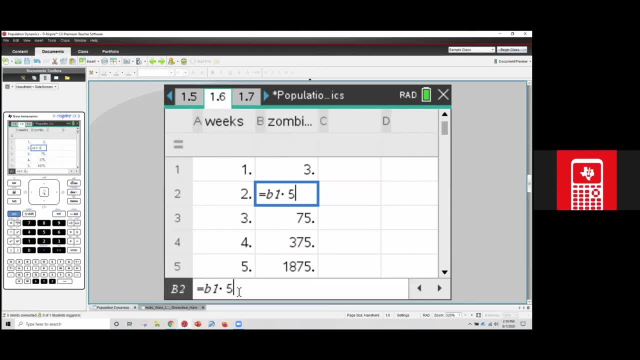 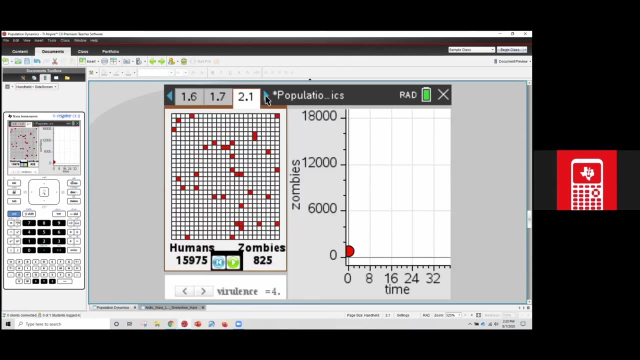 And so by manipulating those values in those equations, you get to see A little bit more of what's going on, And so hopefully, as students, can Get a better computational Understanding of what's happening within that data. With logistic growth It gets a little bit more complicated. 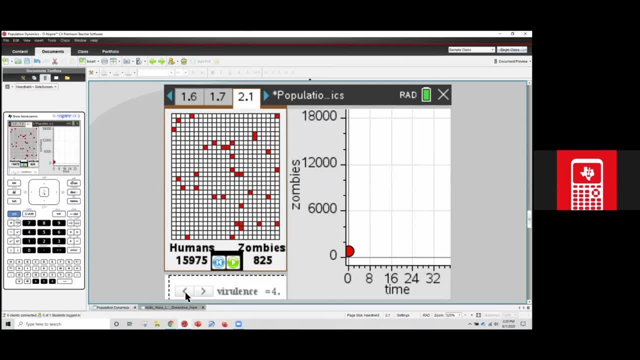 But we've got a lot of data here Which shows how the zombies are increasing, And so we're seeing numbers in those numbers And we're also seeing them that carrying capacity, And so when we are using our zombies. So let me play our zombies. 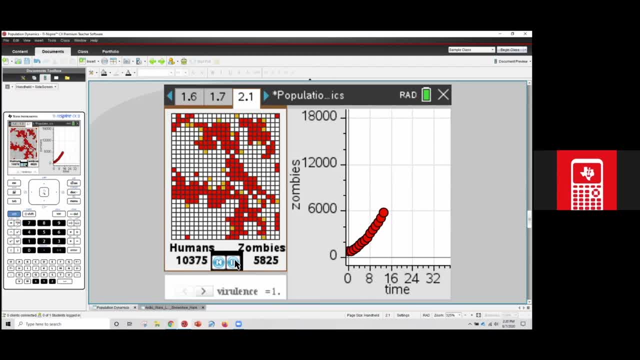 So we've got two visual representations, A data table- I'm sorry, Not a data table- A graph on the right That's showing how the zombies are increasing over time, but on the left, we're also getting data too. Well, it looks like. it looks like the red squares are people who have been infected and thereby turned into zombies. 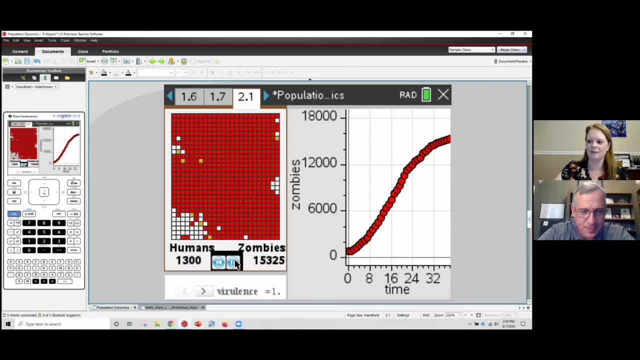 Yeah, So that you know it's not a traditional data table or graph, but it is providing information about what's happening, And so giving giving students access to different ways of representing information is also a very valuable tool. Seeing that those squares turn red? not all of them. 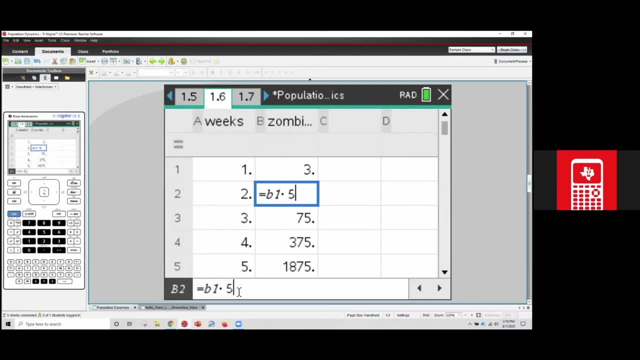 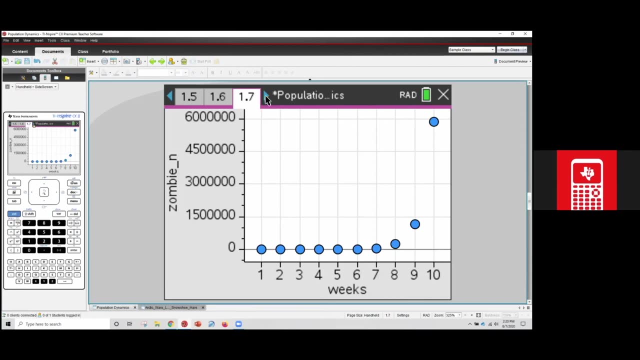 how the rate changes, And so by manipulating those values in those equations, you get to see a little bit more of what's going on, And so hopefully students can get a better computational understanding of what's happening, And so we can also see what's happening within that data. With logistic growth it gets a little bit. 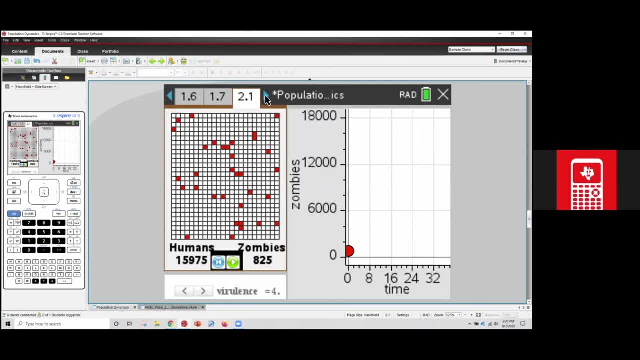 more complicated because we're adding in that carrying capacity And so when we are using our zombies, so let me play our zombies here. So we've got two visual representations. We've got a data table- I'm sorry, not a data table- A graph on the right that's showing how the zombies are. 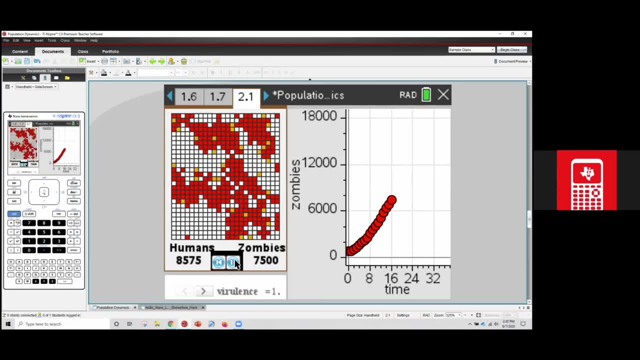 increasing over time. But on the left, we're also getting data from the zombies, So we can see how the zombies are increasing over time. But on the left, we're also getting data too. We're having these red squares up here. And what are those red squares representing? Eric. 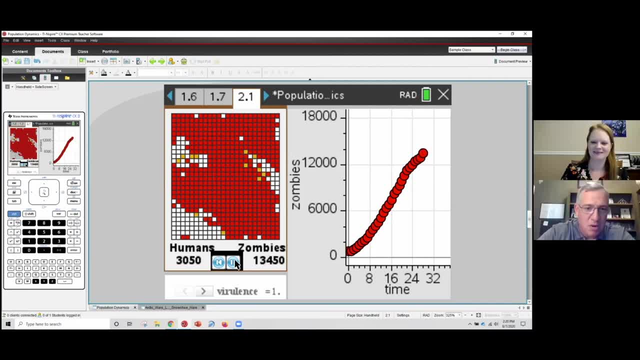 Well, it looks like. it looks like the red squares are people who have been infected and thereby turned into zombies. Yeah, so that you know, it's not a traditional data table or graph, but it is providing information about what's happening And so giving, giving. 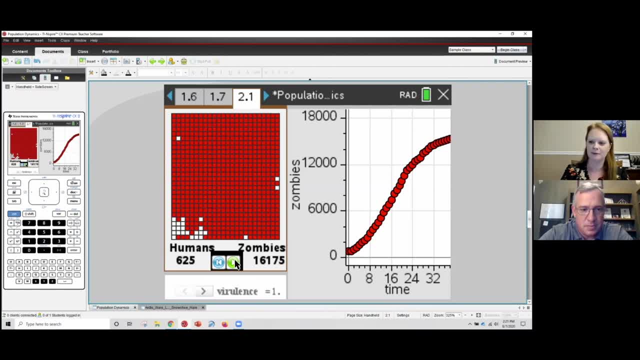 students access to different ways of representing information is also a very valuable tool. Seeing that those squares turn red- Not all of them, There's still some humans left, but our population, Oh, so are those. So those white squares that are left, those are the healthy humans, right? 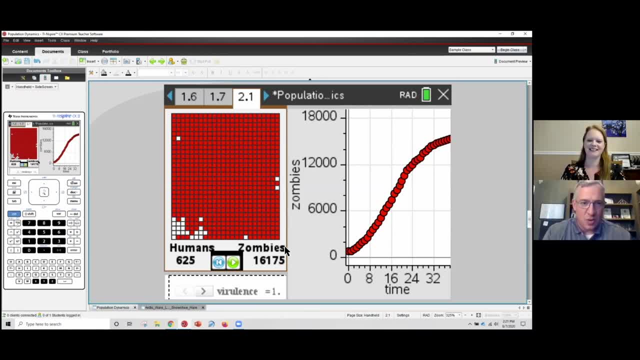 Mm-hmm. so that's, Those are the only resources that are left in that population right And there's not a lot left. So the zombies have kind of leveled off off. They've reached that max and reached that carrying capacity because there aren't as many. 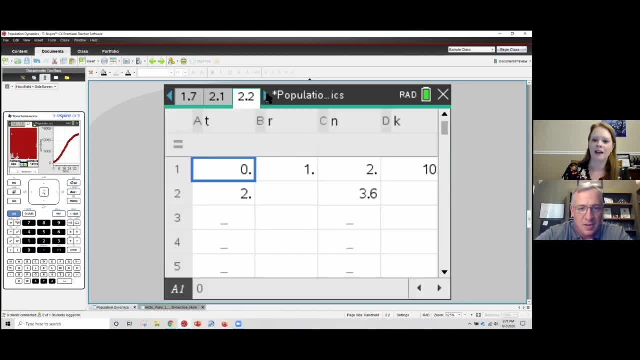 resources there for them. and so what? I again using a spreadsheet, I've got time, and so to put time in here, I've already pre-populated it to make it easier on myself, but I added the equation a1, which is time zero plus two. so I'm increasing that time increment by two, and so I can then drag. 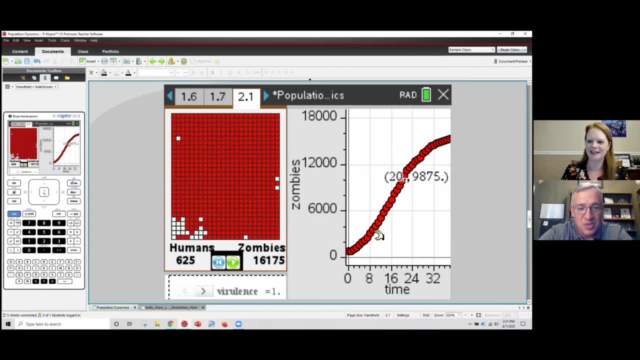 There's still some humans left, but our population here, Oh so are those. so those white squares that are left, those are the healthy humans, right. So that's, those are the only resources that are left in that population, Right, And there's not a lot left, So the zombies have kind of leveled off. 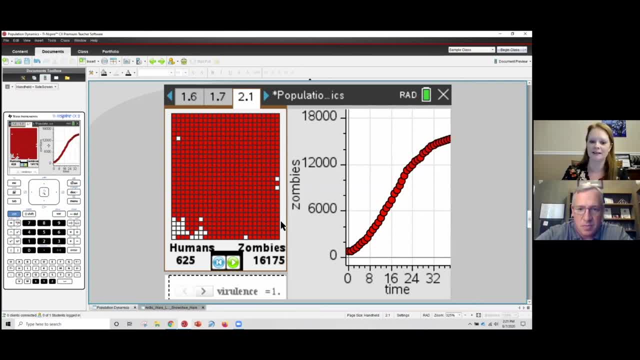 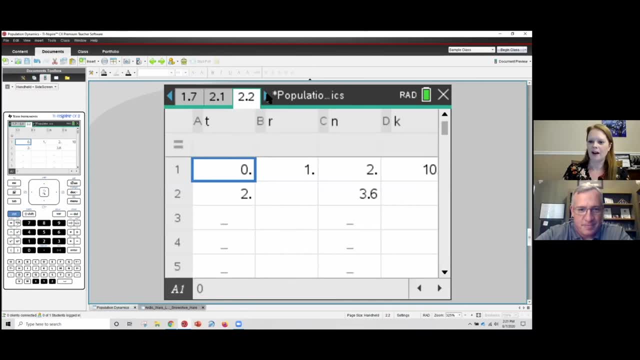 They've reached that max and reached that carrying capacity because there aren't as many resources They are for them. And so what? I again, using a spreadsheet, I've got time, And so the kid put time in here. I've already pre populated it to make it easier on myself. 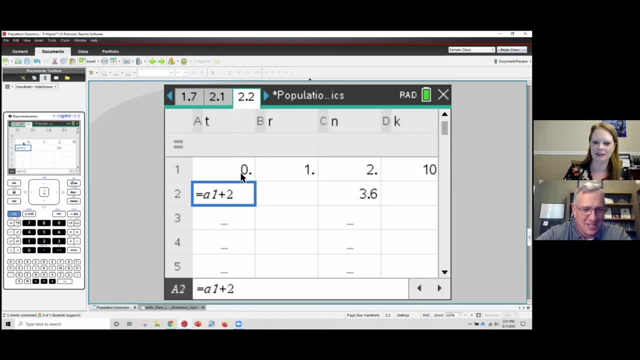 But I added the equation a one, which is time zero plus two. So I'm increasing that time increment by two And so I can then drag that down. So let's do two, maybe about 20 timescale. So whether we're talking about weeks or seconds or months, where we have to decide that we have a rate of one right now, 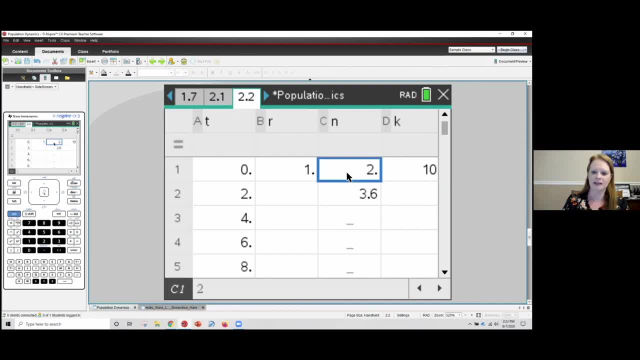 And then our N is going to be our C1, which is our initial population times F1. And I'm going to change this over to the computer view on the teacher software, just because it gives a better idea of what's going on The spreadsheet. 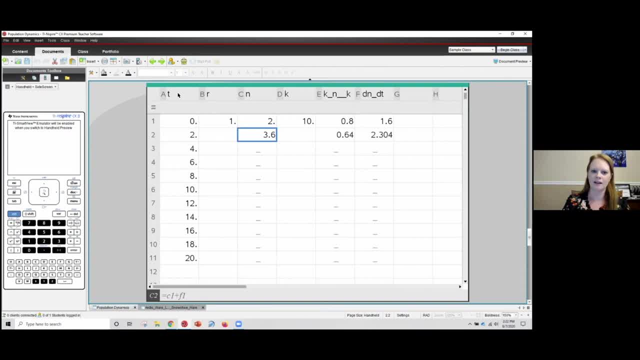 And so you can see what's going on up here. So I've got time, which is T. We've got R, which is that our max rate. We've got N, which is our population number, Our K, which is our carrying capacity. This is our, that that proportion, K minus N over K, And this is our population growth of DN over DT. 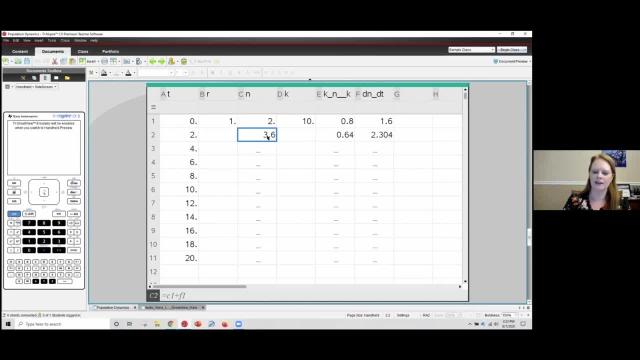 And so for this one, for N, we have to calculate it with our C1 plus F1.. So we have to add in our population from F1 over here as it increases for each increment, each time increment, we have to look at our population growth And so we're going to add that in And so we can start looking at if our 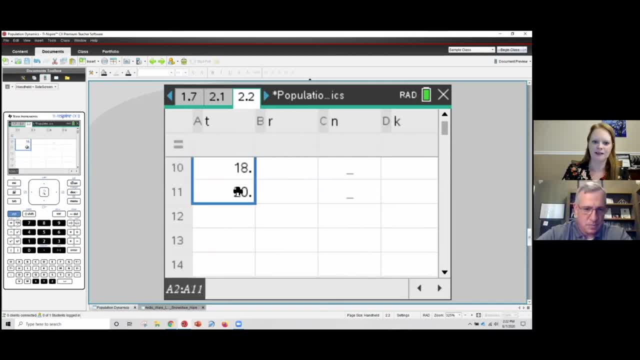 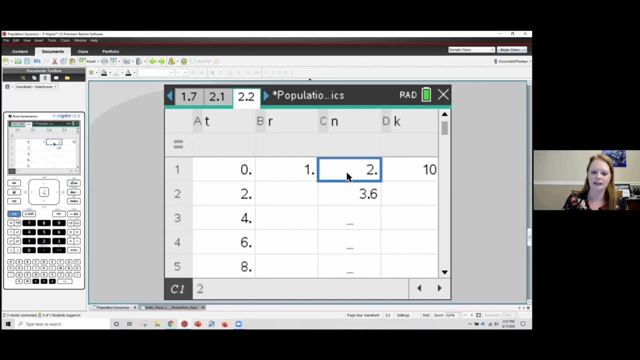 that down. so let's do to, maybe about 20 timescale. so whether we're talking about weeks or seconds or months, we have to decide that We have a rate of one right now, and then our n is going to be our c1, which is: 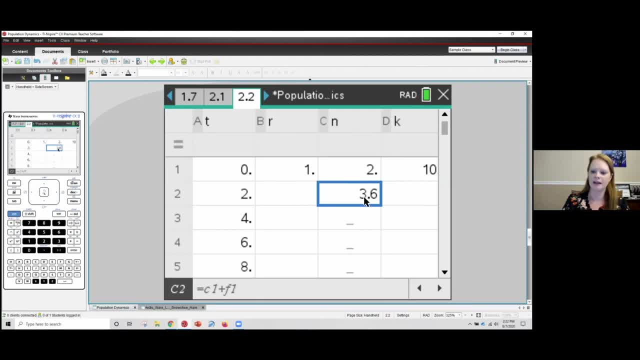 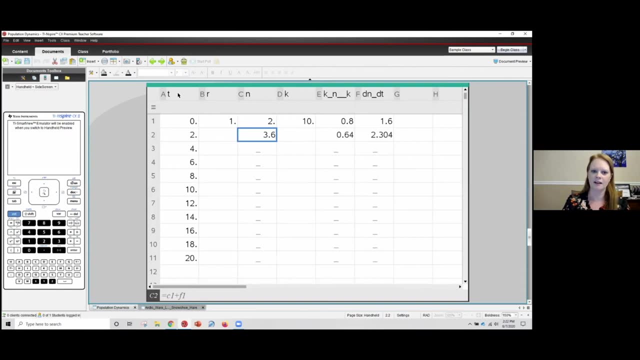 our initial population times, f1, and I'm going to change this over to the computer view on the teacher software, just because it gives a better idea of what's going on in the spreadsheet and so you can see what's going on up here. so I've got time, which is t. We've got r, which is that r max. 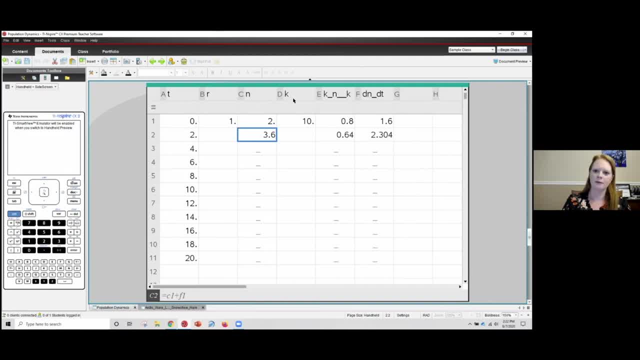 rate. We've got n, which is our population number, our k, which is our carrying capacity, This is our that proportion, k minus n over k, and this is our population growth of d n over d t. and so for this one, for n, we have to 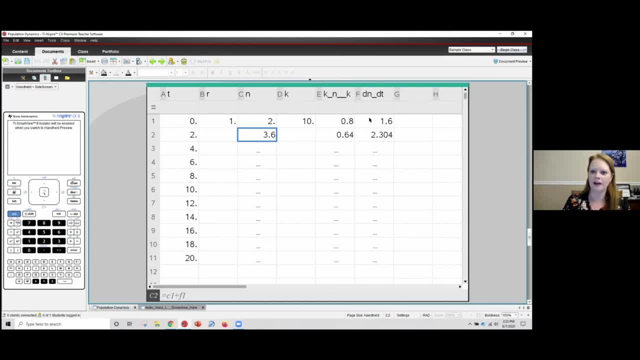 calculate it with our c1 plus f1.. So we have to add in our population from f1, over here as it increases. for each increment, each time increment, We have to look at our population growth, and so we're going to. 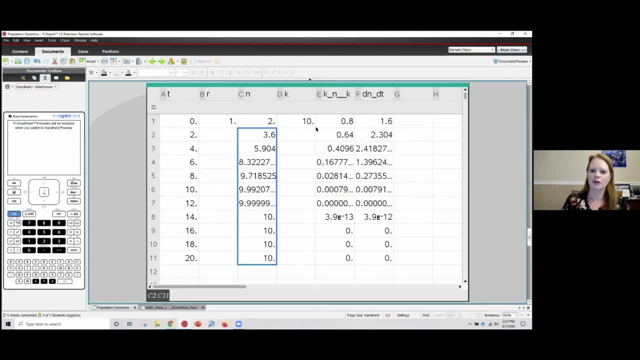 add that in, and so we can start looking. if our rate is constant and our carrying capacity is at 10, this is what's going to be going on, and so we can see that our rate is increasing. initially, so 2 is much higher than 0, and then what's going to be happening down here is that it's 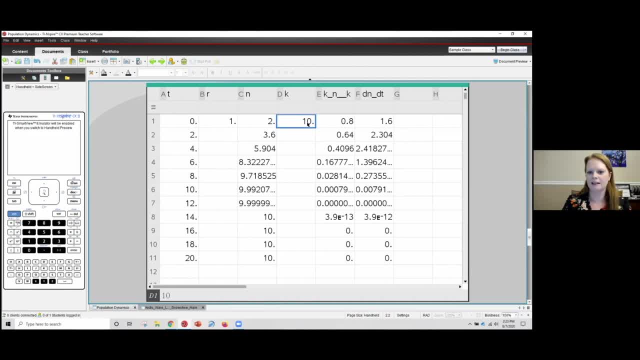 rate is constant and our carrying capacity is at 10,. this is what's going to be going on, And so we can see that our rate is increasing. initially, So two is much higher than zero, And then what's going to be happening down here is that it's going to be leveling out, And so we can graph this again and see what's happening. 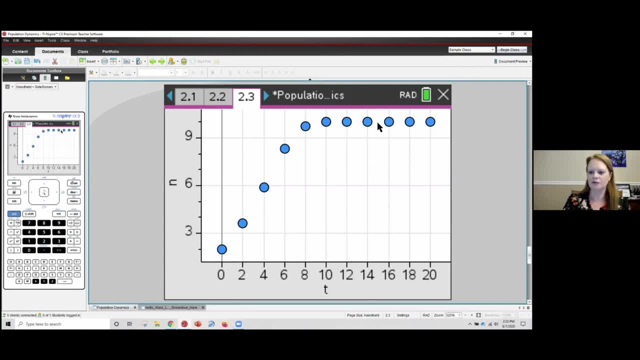 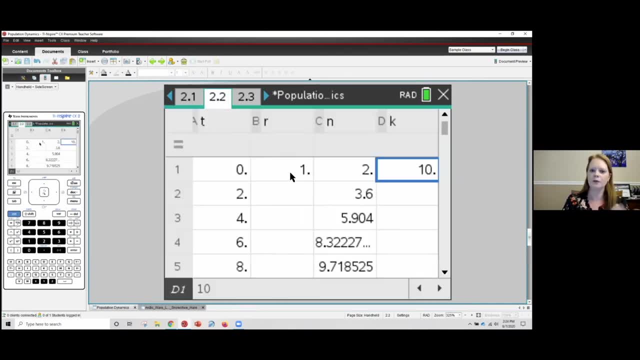 So we can see this increase and then, where it's reached, that carrying capacity, and then not being able to fluctuate much more, And so by playing around with either the rate or the carrying capacity, you can see fluctuations in the population. So let's make the carrying capacity now. 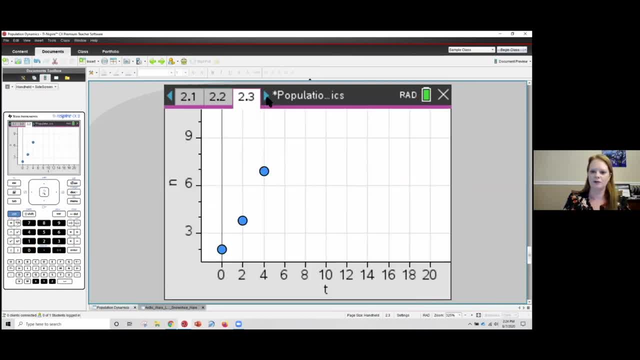 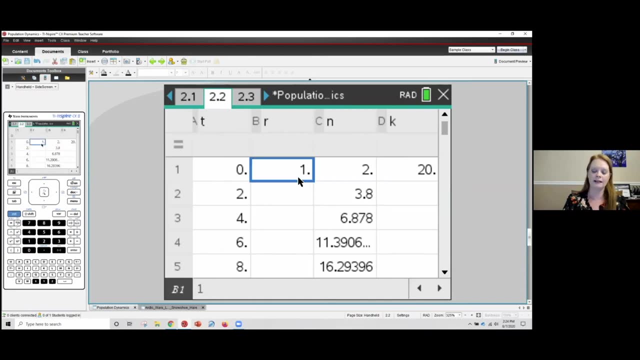 20 and see what that does to our graph. And because we are now at a different graph, we're going to need to zoom in to our data And see, now that our population increases and then levels off and we can change our rates to, let's say, maybe three, and what happens. And so here this looks messy. 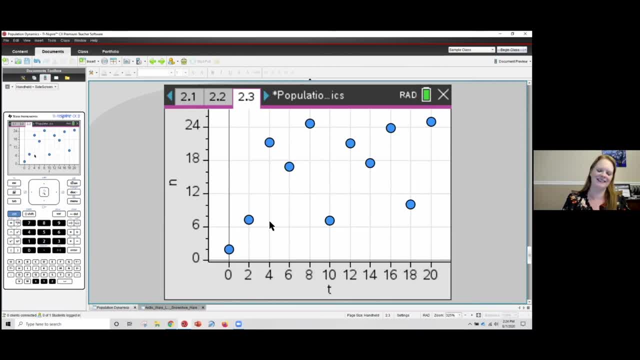 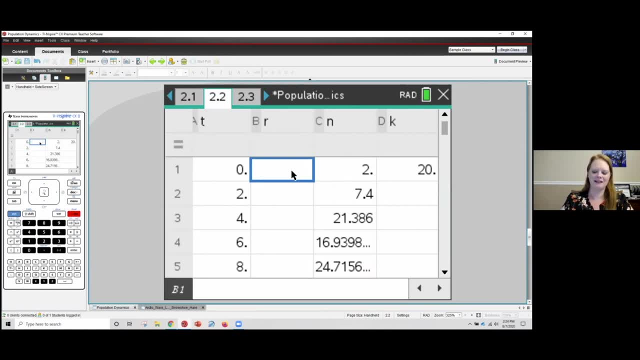 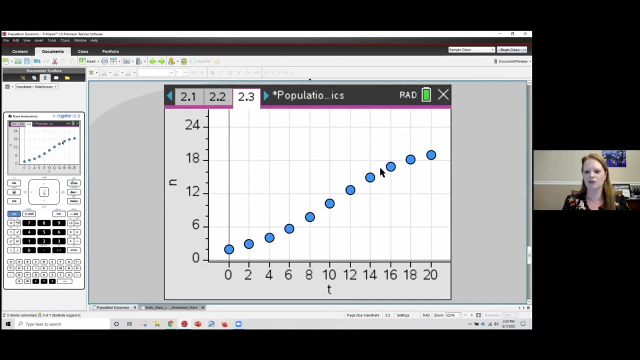 Let's see if it improves any here. All right, that looks very weird, But we can go back and change it back to, let's say, what happens at 0.5, And then we get this kind of Not a steep curve, It's a little smoother. And let me just make sure that all of our data is in there to make sure that we get a better representation of. 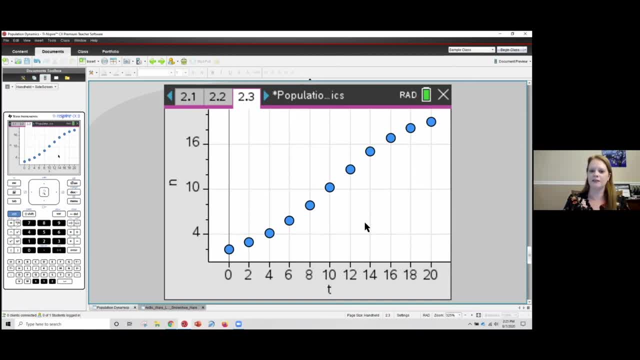 And we were looking at very different curves based off of that rate and our carrying capacity. So by building a spreadsheet and getting kids to understand what those values represent in each of those categories And then being able to manipulate those categories, they can see how that population fluctuates and what those 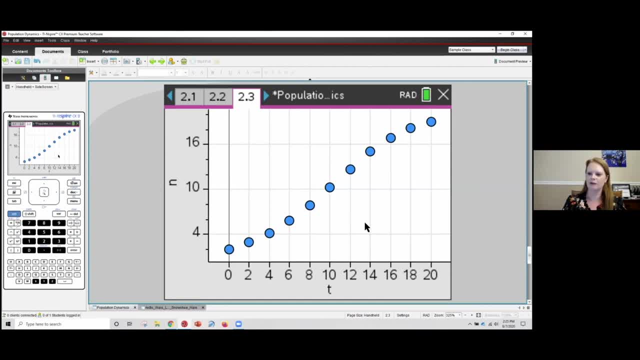 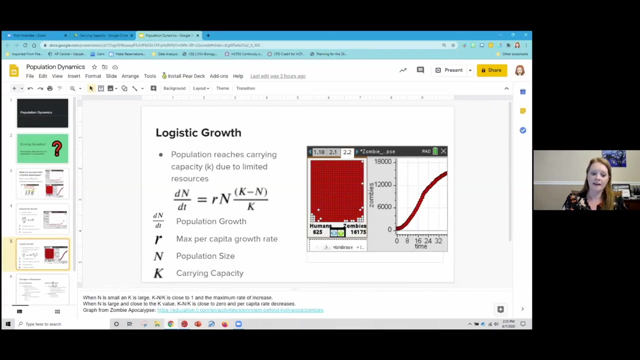 How carrying capacity is really important in a population, looking at what those resources are, whether they're available and how the numbers of those organisms affect what's going on within that ecosystem. And so having that mathematical and computational thinking, relating it back to the data that they're given, is really important, And from there they can identify and 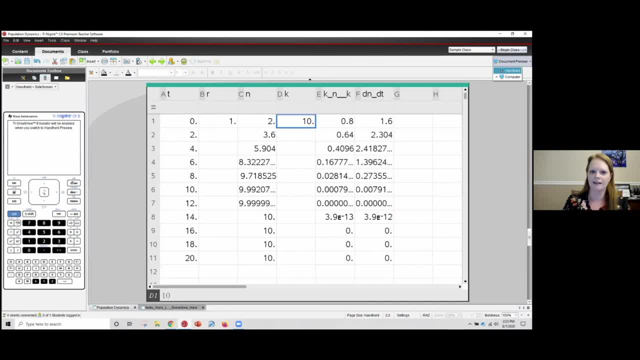 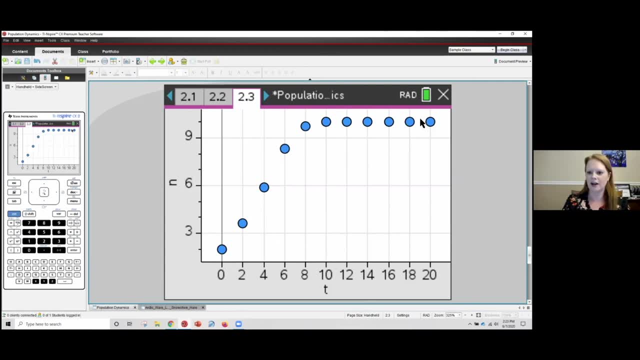 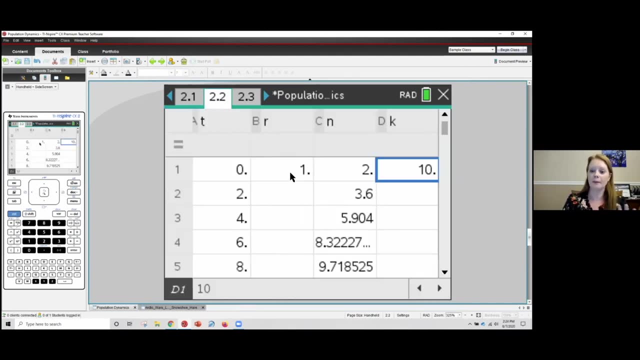 going to be leveling out, and so we can graph this again and see what's happening. so we can see this increase and then, where it's reached, that carrying capacity and then not being able to fluctuate much more, and so, by playing around with either the rate or the carrying capacity, you can see 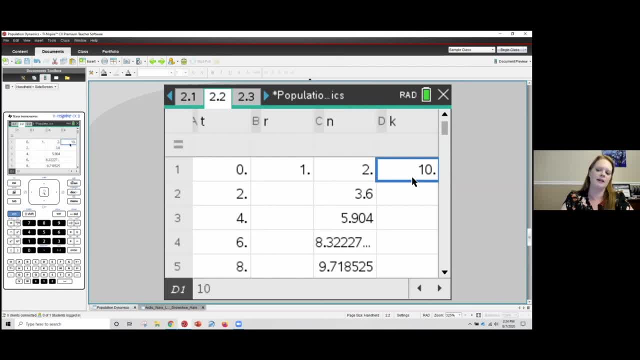 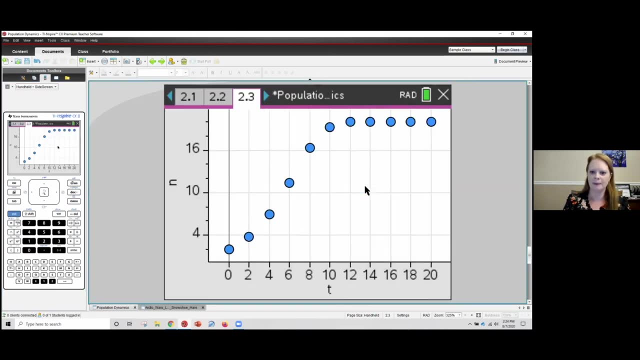 fluctuations in the population. so let's make the carrying capacity now 20 and see what that does to our graph. And because we are now at a different graph, we're going to need to zoom in to our data and And see now that the rate is increasing. an increase in the carrying capacity is a pretty significant one. 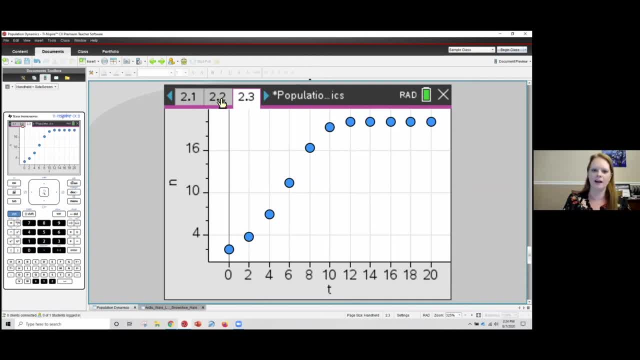 that our population increases and then levels off, and we can change our rate to, let's say, maybe three, and what happens? And so here, oh, this looks messy, Let's see if it improves any here. All right, that looks very weird. 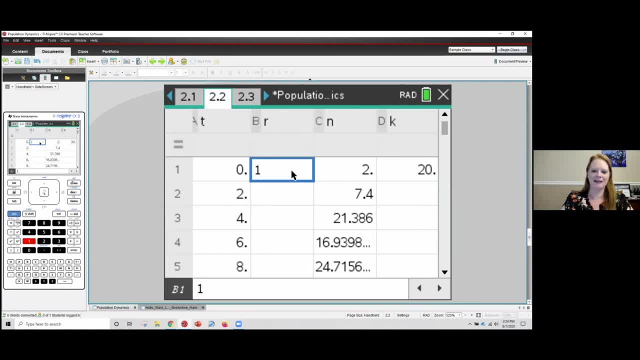 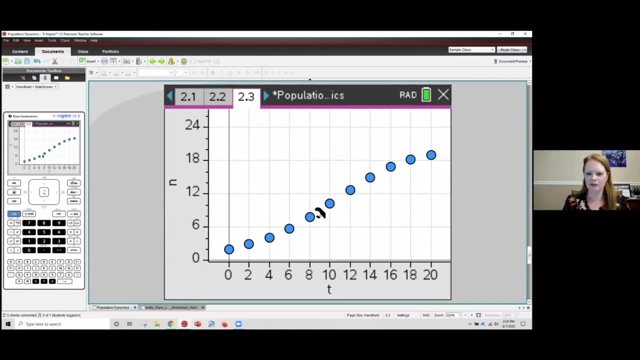 But we can go back and change it back to, let's say, let's see what happens at 0.5. And then we get this kind of not as steep curve. it's a little smoother, And let me just make sure that all of our data is in there. 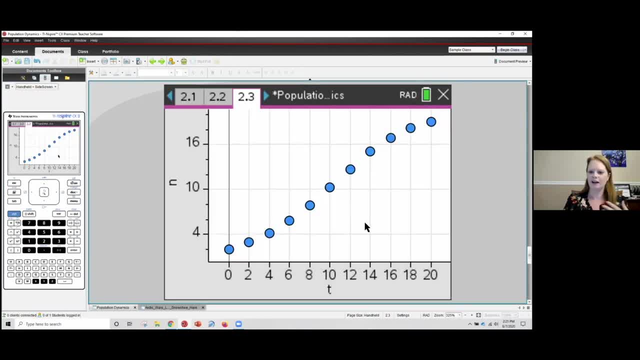 to make sure that we get a better representation of- and we were looking at very different curves based off of that rate and our carrying capacity. So by building a spreadsheet and getting kids to understand what those values represent in each of those categories and then being able to manipulate them. 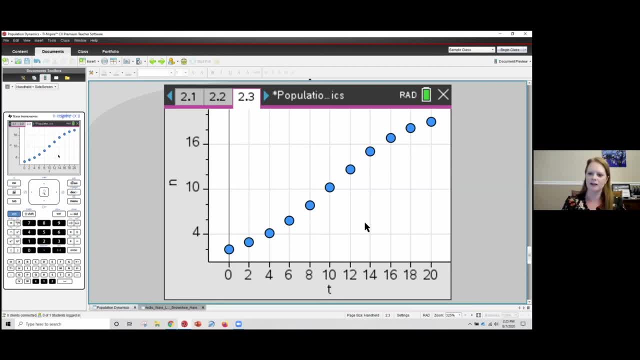 and manipulate those categories, they can see how that population fluctuates and how carrying capacity is really important in a population, looking at what those resources are, whether they're available and how the numbers of those organisms affect what's going on within that ecosystem. 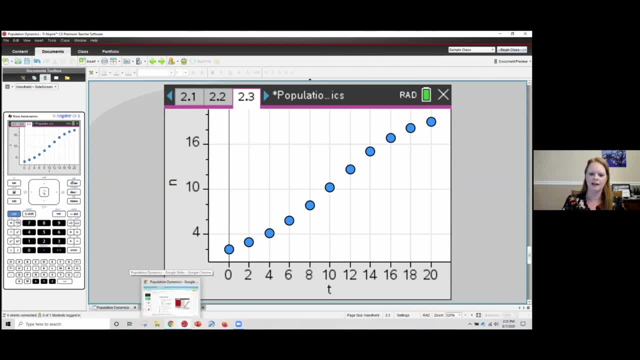 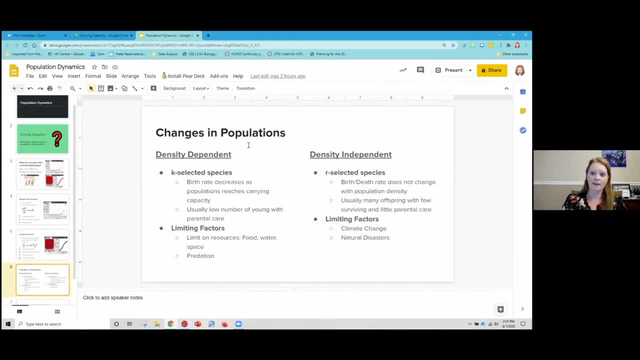 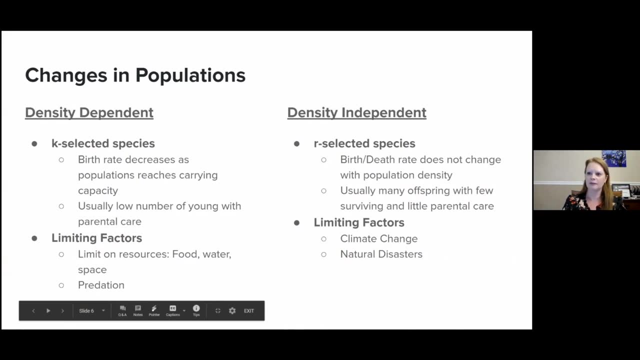 And so having that mathematical and computational thinking, relating it back to the data that they're given, is really important, And from there they can identify and make some connections with the organisms and how those reproductive strategies and organisms are needed, or what am I trying to say? 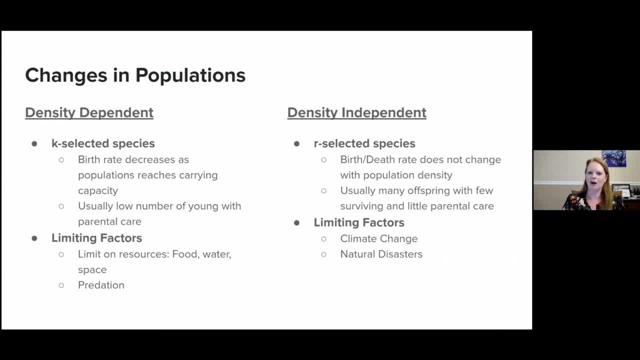 that like how those changes in the populations are caused, whether they're density dependent or density independent, So whether they're K selected species where, like humans, I would assume zombies as well, that they, where the birth rate decreases as the population reaches that carrying capacity. 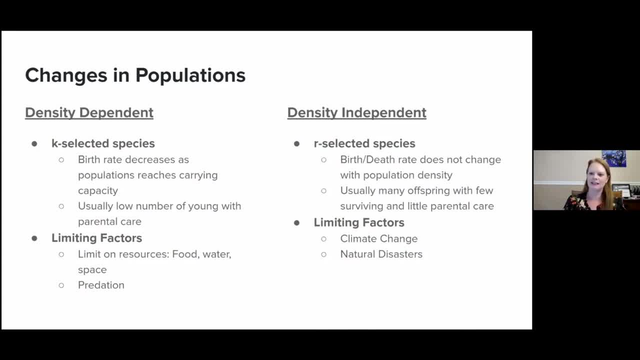 because the death rate increases and that's where the population is normally in and that carrying capacity is fluctuating as around that carrying capacity where the organisms tend to have fewer babies and take care of them longer And those limiting factors are going to be dependent. 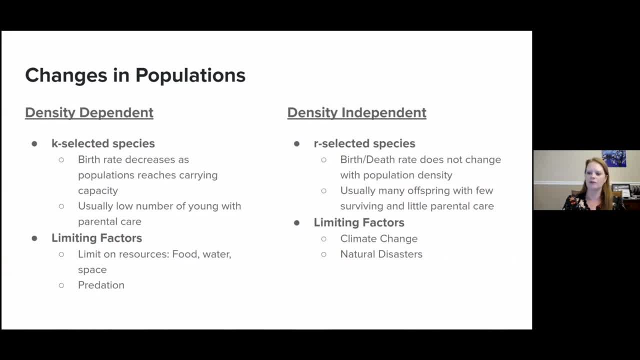 Make some connections with the organisms and how those reproductive strategies and organisms Are or need are. What am I trying to say? that that like how those changes in the populations are caused, whether they're density dependent or density independent, So whether they're case selected species where, like humans, I I would assume, zombies as well. 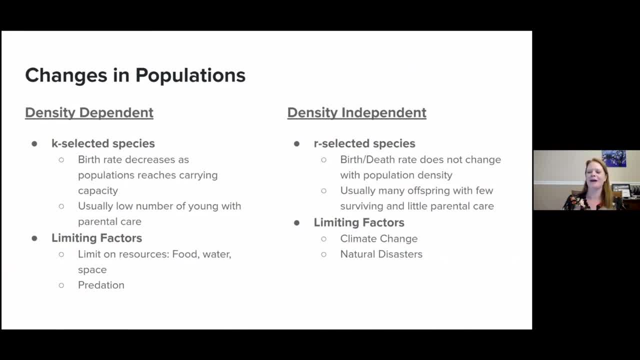 That they were. the birth rate decreases as the population reaches that carrying capacity because the death rate increases And that's where the population is normally in and that carrying capacity is fluctuating And so they're able to control that around that carrying capacity, where the organisms tend to have fewer babies and take care of them longer. 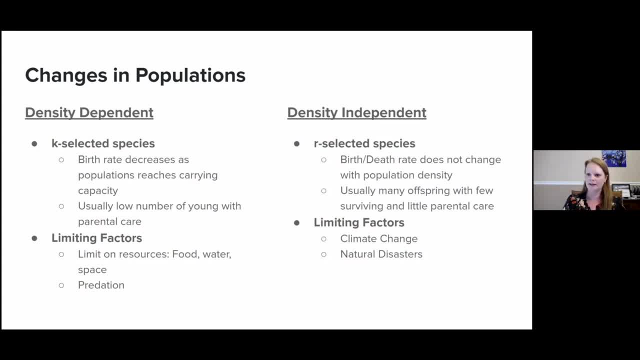 And those limiting factors are going to be dependent on the density of the population, such as food, water, shelter And then predator prey. relationships are really important with that as well, And so with our zombies, They were dependent on their prey, which is healthy humans, And once those were gone, 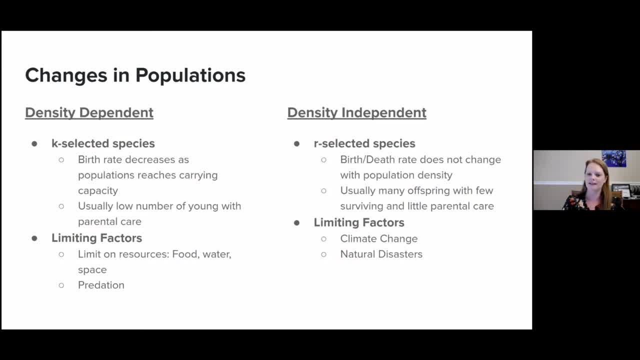 You know, that's where the population decreases, the population reaches its carrying capacity. But then there's also density, independent factors and species, where the birth rate and the death rate changes but it doesn't affect the population density or it doesn't change with the population density And so with those types of organisms. 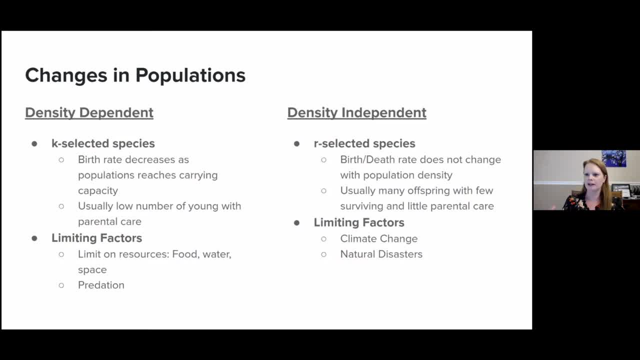 like, I think, a weeds, where you have lots of offspring all at once and then very few of them actually survive to adulthood. and so those limiting factors are density of density, independent, which don't rely on population density, or things like climate change, natural disasters, which will help, which would then fluctuate the numbers based on external factors, not necessarily. 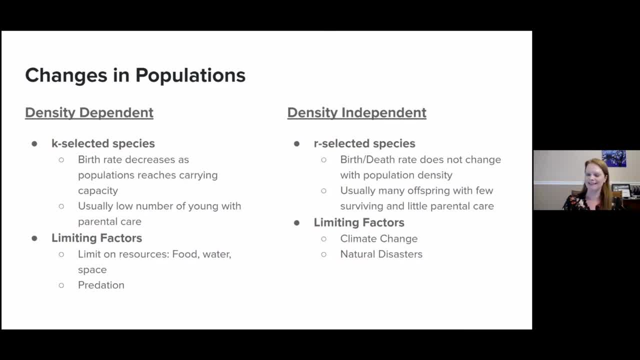 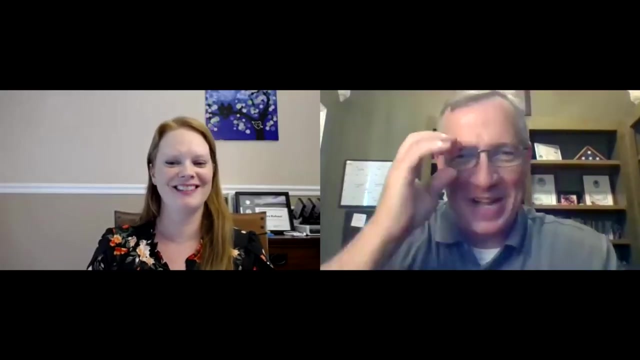 density, And so using zombies is a fun way to kind of relate to some of these concepts and give students an energetic way of learning about population dynamics. Yeah, I've always heard that students. a lot of times after lunch they kind of turn into zombies. I don't know if that's true or not, but 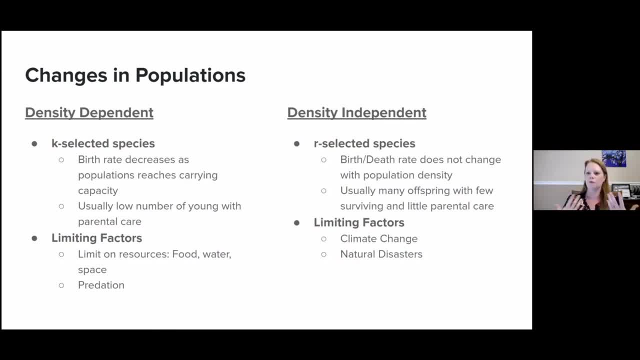 on the density of the population, Such as food, water, shelter and then predator-prey. relationships are really important with that as well, And so with our zombies. they were dependent on their prey, which is healthy humans, And once those were gone, 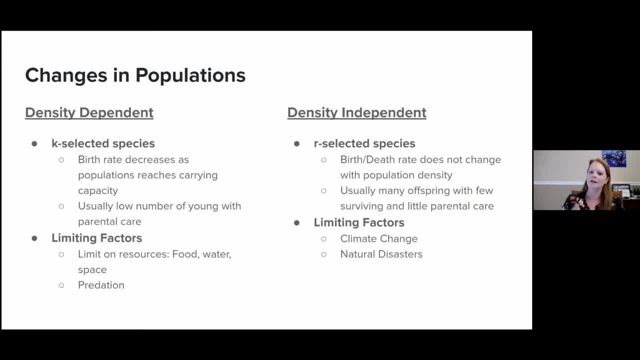 that's where the population reached carrying capacity. But then there's also density, independent factors and species where the birth rate and the death rate changes but it doesn't affect the population density or it doesn't change with the population density And so with those types of organisms. 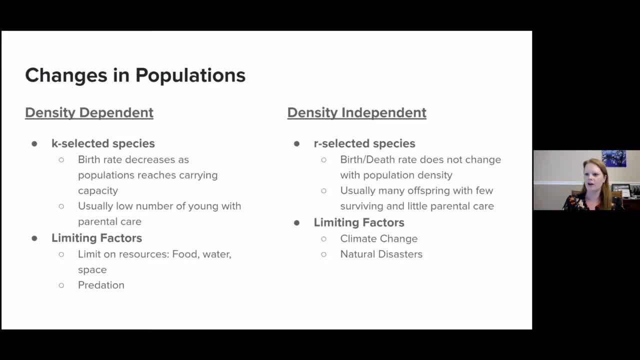 like I think of weeds, where you have lots of offspring all at once and then very few of them actually survive to adulthood. And so those limiting factors of density independent, which don't rely on population density or things like climate change, natural disasters, 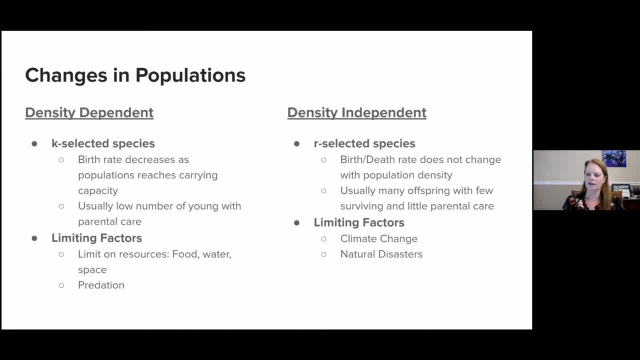 which would then fluctuate the numbers based on external factors, not necessarily density, And so using zombies is a fun way to kind of relate to some of these concepts and give students an energetic way of learning about population dynamics. Yeah, I've always heard that students a lot of times. 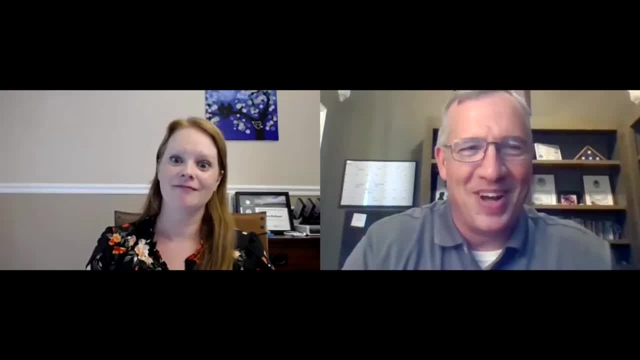 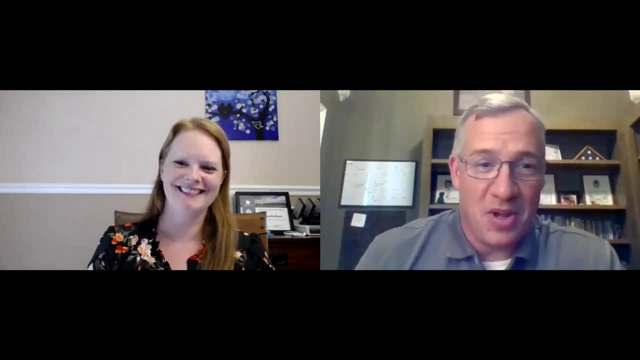 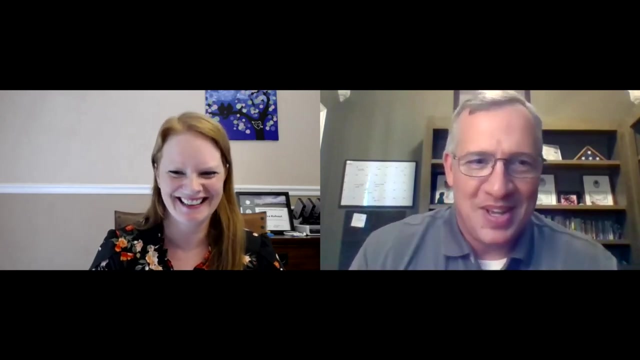 after lunch they kind of turn into zombies. I don't know if that's true or not, but yeah, I've heard stories, Let's just put it that way. So I love this lesson. I thought this was great. I like how you walked us through using a fake organism: zombies. 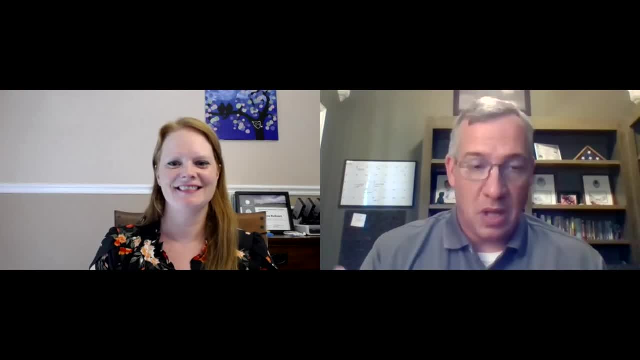 as a way to sort of model a real life relationship. So an organism, a species, can only increase its numbers so much. There's a limit to how much they can increase And that's based on the carrying capacity of the environment, what it can, how much food is available for that. 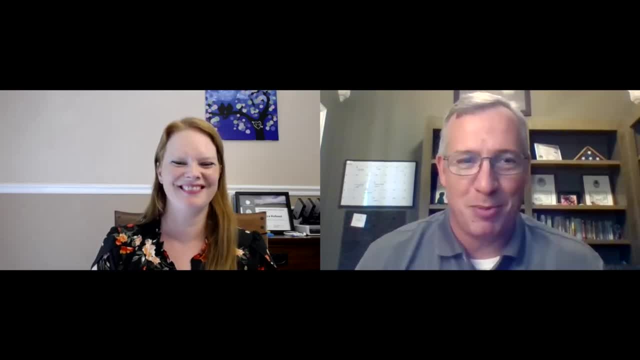 particular species. In this case it was zombies eating humans, which is super creepy, But the example still holds. It still makes sense, So great job. I love the lesson And I've learned a lot about population dynamics and carrying capacity.